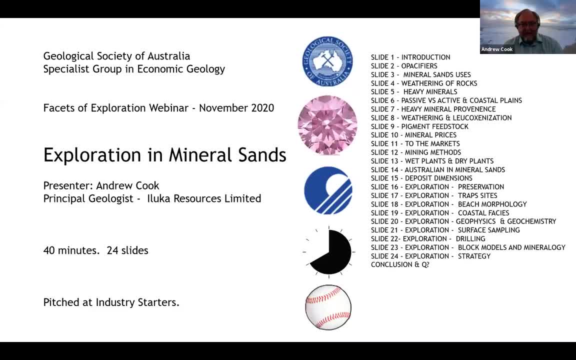 you who are more experienced, I'll be talking about what mineral sands are and why they're sought, where they originate and how their composition varies from place to place. You can all glaze over for a bit while I talk more specifically about the chemistry of 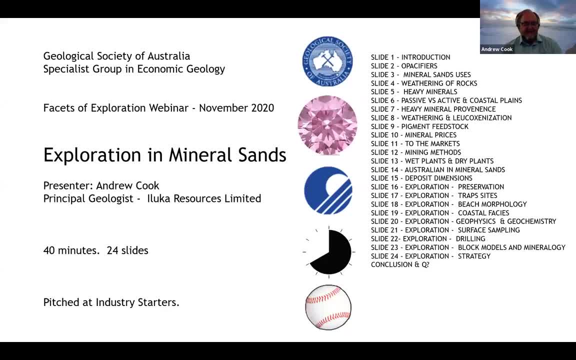 ilmenite and what the different variations are used for. I'll talk a little bit about mineral sand economics, perhaps about the dimensions of deposits required and how the mixes and assemblies of heavy minerals is important. A little bit about mining methods and how the minerals are separated. 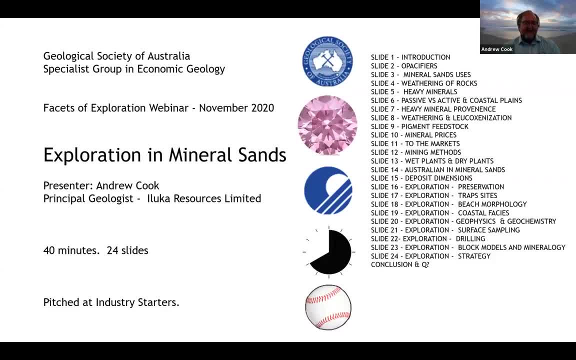 then back up to geological settings at the end and some of the techniques we use. Hopefully we'll be looking at about 40 minutes. You should get to know enough about mineral sands to be dangerous by the end, or perhaps enough to go out and find your own ore body. Just make sure. 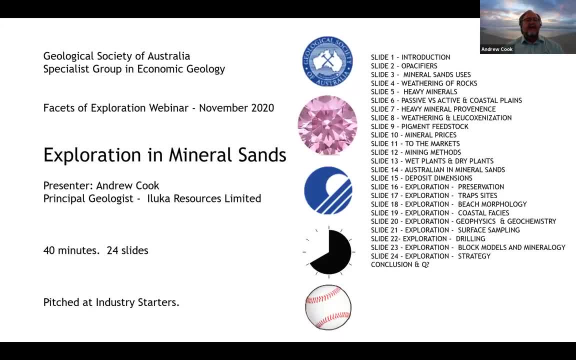 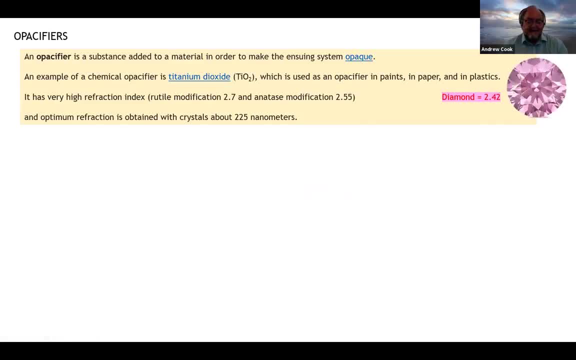 you bring it to Eulika first. Facets of exploration is a good title because facets as reflectors of light and crystals. it's very appropriate descriptor in relation to mineral sands. Refractive indices and the scattering of light is what mineral sands is all about. 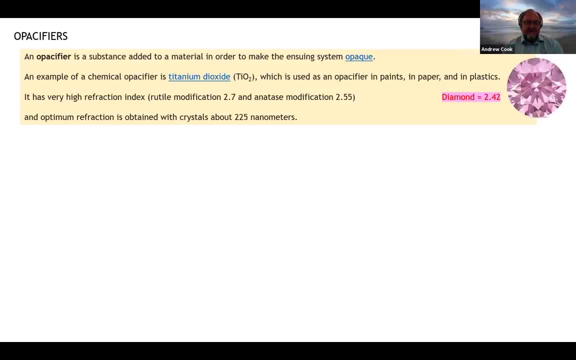 feedstock minerals to the chemical industry, and the main chemical industries that use mineral sands are the paint, paper filler and ceramic glaze industries, and in each of those the various mineral products we supply are used as opacifiers. Opacifiers are minerals that, because of their 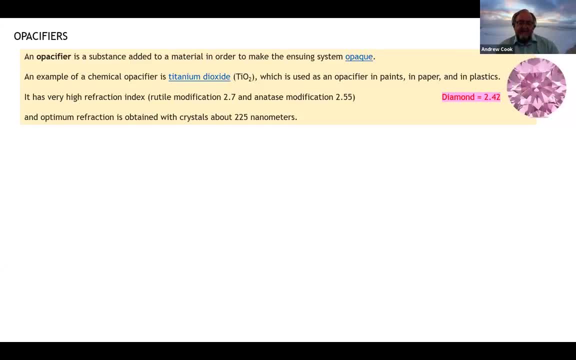 high refractive index are able to scatter light and reflect it back, and by so doing they hide the surface underneath Exactly like that. So titanium, zircon: they're both adjacent group for elements on the periodic table and they both have these high refractive indexes, higher even than diamond. 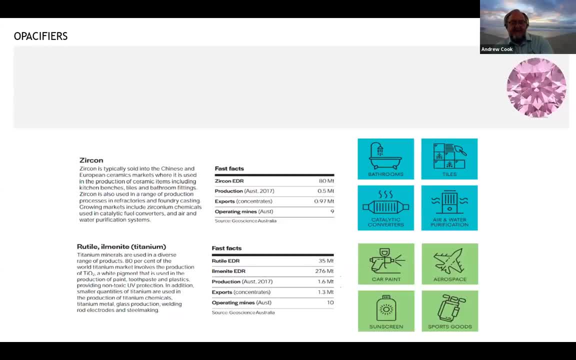 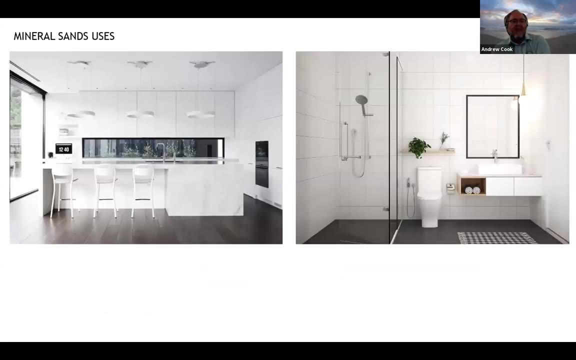 And the titanium and zirconium minerals are the chief constituents of the field called mineral sands. There's a few icons there showing some of the basic uses of the minerals, but we'll get into a bit more detail. So you think titanium, zircon, you know high-tech metals, aerospace? 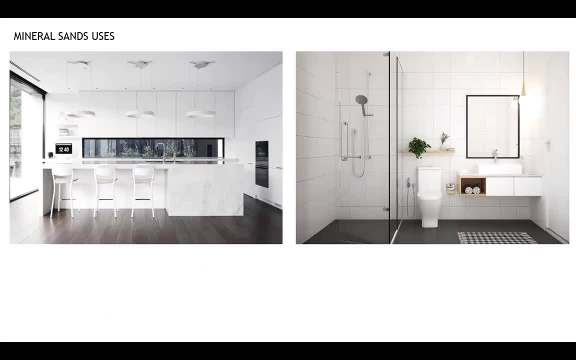 nuclear reactors, you know, maybe golf clubs, artificial equipment, you know things like that. So you think titanium, zircon, you know things like that. But in fact the bulk of mineral sands is used for paint and paper and coatings. It's probably only about less than 10 percent of titanium that actually makes it to titanium metal. 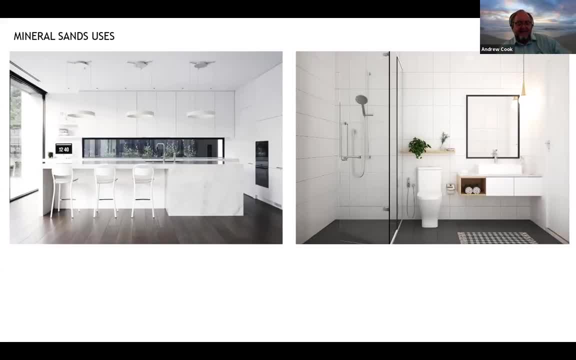 and an even smaller proportion of zirconium that ends up as the metal. But if you stop and look around you, or maybe your kitchen or your bathroom or just the walls in the room you're in, you'll see that these coatings are pretty much everywhere. 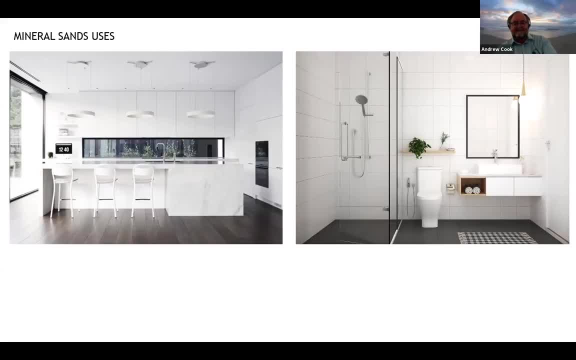 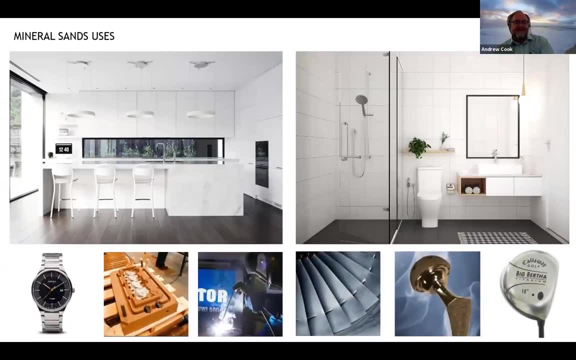 and you're probably in contact with titanium dioxide almost every day. There is, you know, a bunch of other uses too. There is some that goes to titanium metal. It's used for things like watches and golf clubs and artificial hips or turbine blades. The mineral rutile is used as a flux on welding rods and 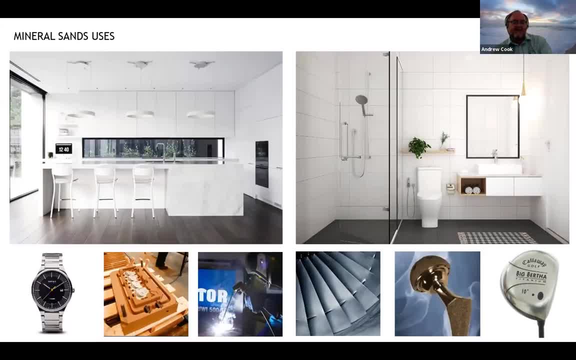 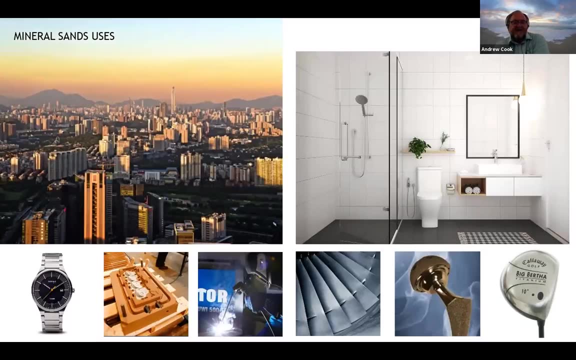 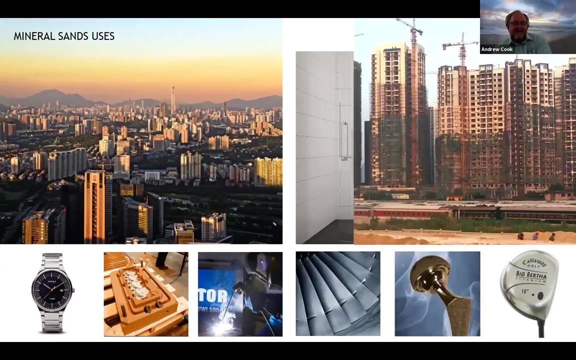 zircon is also well used for as a casting sand for casting metal, But in general the demand for mineral sands is closely linked to construction, welding, building, and it's driven by the increases in urbanizations that are going on, This worldwide drift of people from the country into the cities. 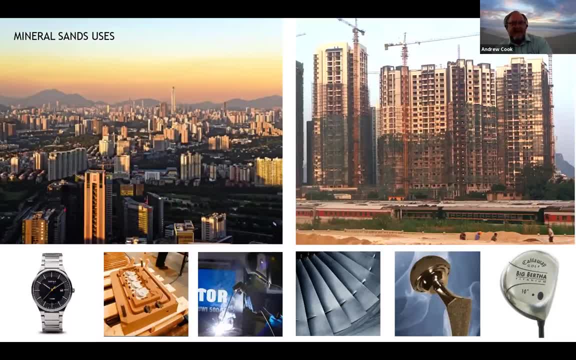 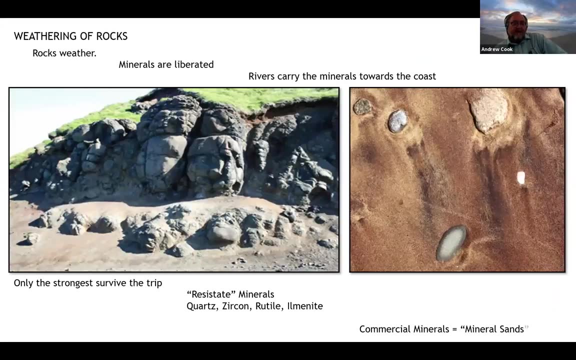 quite good for mineral sands. Those new cities all need paint, they need tiles and people want bathrooms, lots of bathrooms. So that's the minerals. Where do they come from? and what's the sand part of the story? Well, to match the humble uses most mineral sands have a 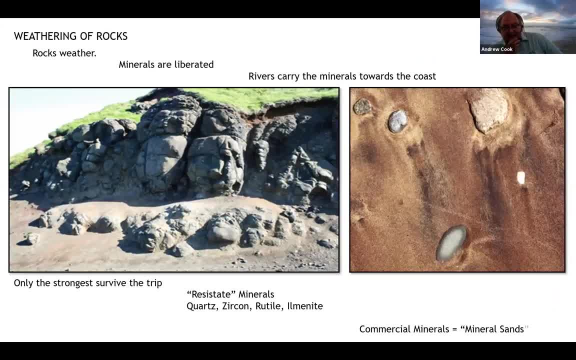 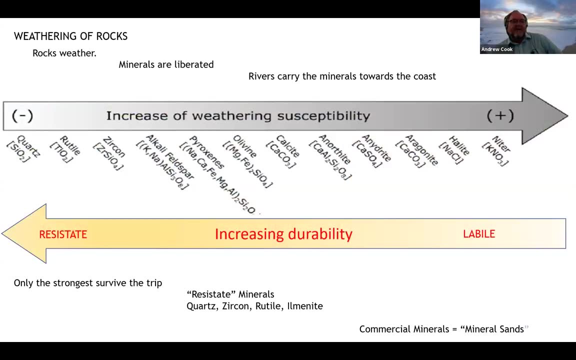 pretty ignominious beginning, and by that I mean the breakdown, the decomposition, the decrepitation of rocks, the weathering of rocks to detritus. Those who remember their basic geology will probably recognize the Goulditch tables of mineral stability and you'll see that not all minerals are equally stable in the 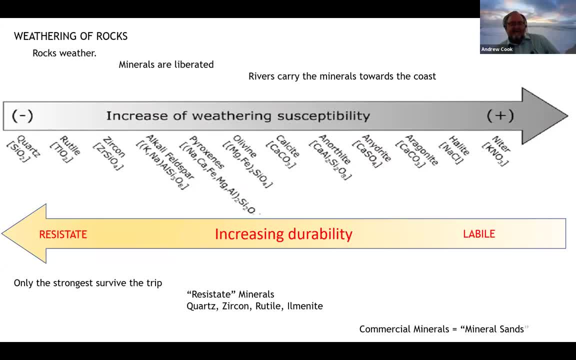 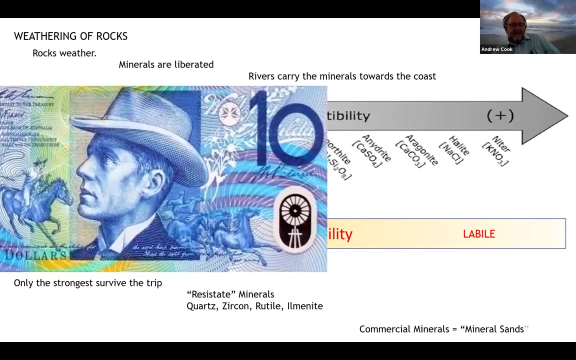 weathering environment. Some disappear quite quickly, fading away to ghostly clays and the likes, but others, the more resistate and durable minerals. they survive and they are washed out of the rocks and travel down rivers and eventually find resting places in new sediments. and you know, like the man from 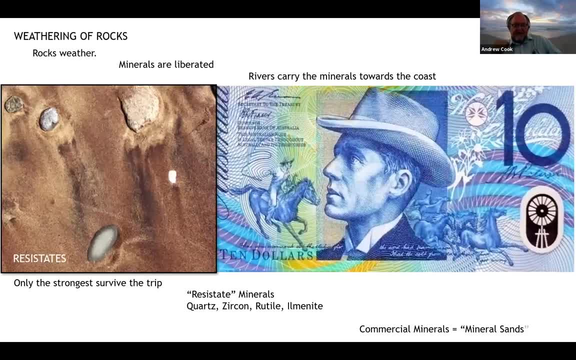 snowy river. the resistate minerals are there riding with them at the end as sand particles. So we have this catchphrase for these minerals, which is mineral sands. Ten dollars, by the way, is is coincidentally around about the in-ground value where mineral sand starts to be of commercial interest. 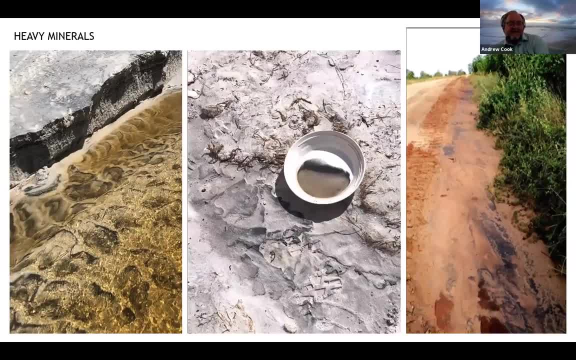 The other thing about mineral, sand minerals, the zircon and ilmenite titanium oxide minerals, is that they're actually heavier than most of your sand And this higher specific gravity allows them to be concentrated when they travel, you know, by the agents of wind and water and waves. 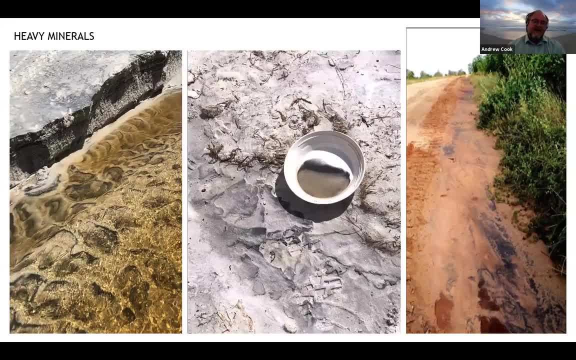 and chiefly through the, the winnowing away of the lighter sand minerals, the quartz and the like. So you know we we often hear mineral sands extended to heavy mineral sands. here's some pictures I took from WA beaches just last week and I think one from Sri Lanka just 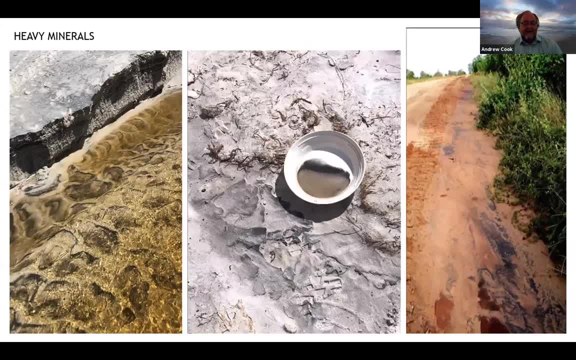 very rich in mineral sands. you'll see in the middle there the white plastic pan. that's our chief tool of trade. there's not much use for hammers in mineral sand exploration Now. these minerals have traveled down rivers and sands and they've been used to transport minerals. 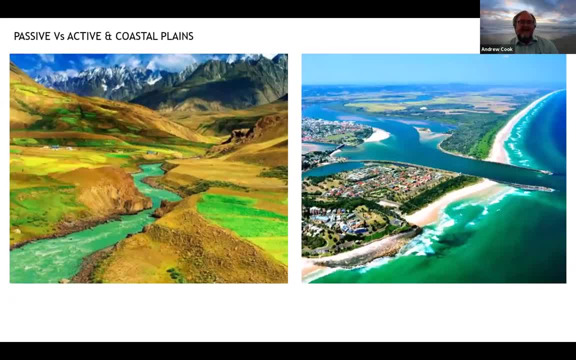 They've traveled down rivers onto coastal plains and in so doing they have a chance for the mineral assemblage to mature. and with coastal plains come coasts, and on coast, waves of the seashore are the most effective winnowers of the heavy minerals. 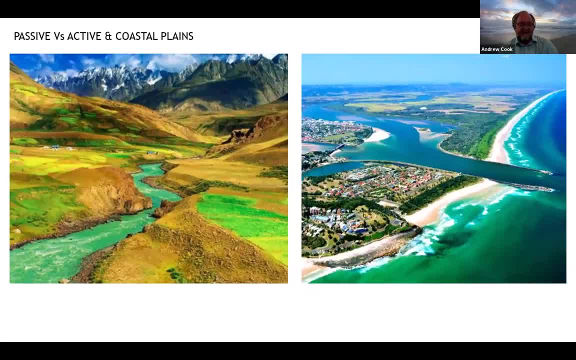 So the best places to find mineral sand deposits are actually, as beach placer deposits. But the trip they've made is important. Short rivers deriving from uplifted tectonically active mountain ranges, Like on the left, there have rapid erosion and short travel and they give you. 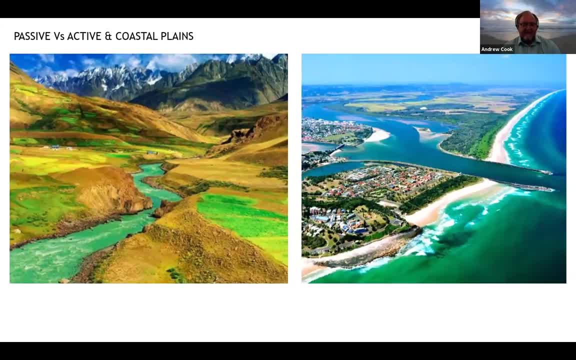 a mix of minerals which has had little chance for the more resistate components to dominate in the heavy mineral assemblage. They're often rich in what the industry calls trash minerals, things like amphiboles, metamorphic minerals like kyanite, staurolite and silimanite. 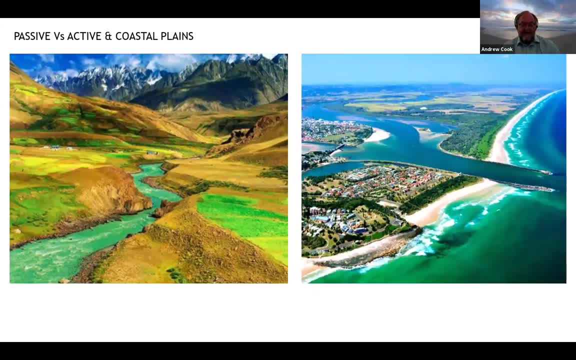 And since these orogenic belts are often used to transport minerals, they're often used to transport minerals. And since these orogenic belts are often used to transport minerals, they're often used to transport minerals. In volcanic there's quite commonly a lot of magnetite and titanomagnetite. 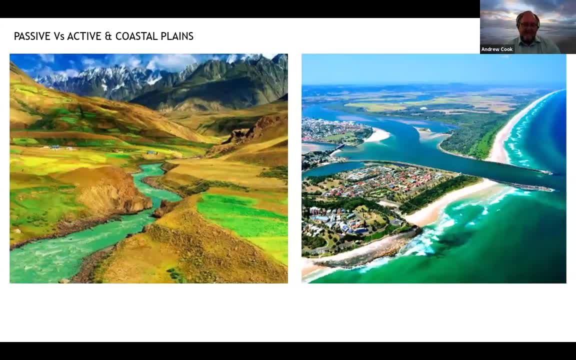 which is all there diluting the minerals we want and it's not readily saleable. Passive continental margins, on the other hand, where slow long rivers deliver minerals onto broad coastal plains with flat, stable coasts, are more likely to be the places where you'll have heavy mineral assemblages that. 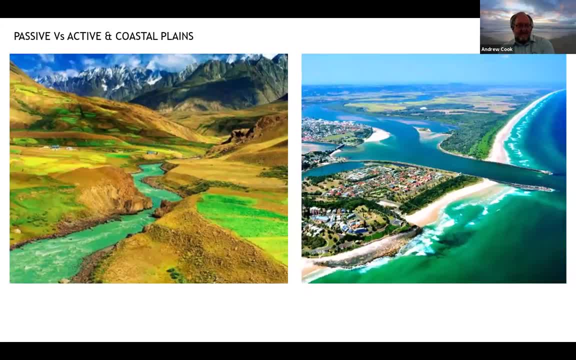 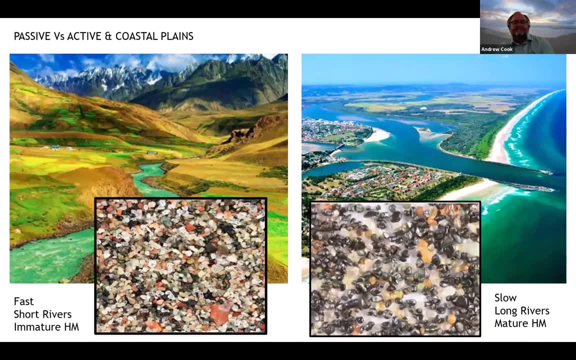 have matured by progressive weathering or abrasion away The. You can see a couple of micro pictographs to illustrate the changes you'll see. In the shot on the right there's a lot more rutile and some of the coccine in there. 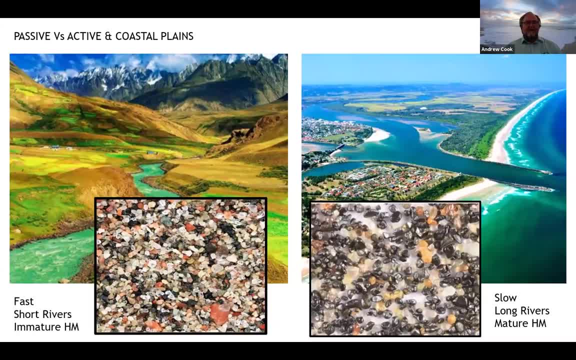 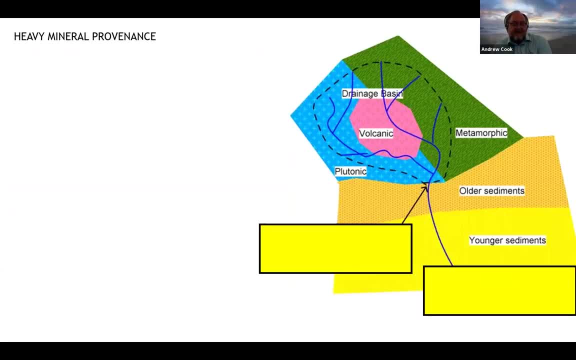 probably a bit of zircon, but you know a more mature assemblage. Now the assemblage really depends upon the source rocks. different rock types will affect the makeup of the heavy minerals that derive from them. Silmanite is perhaps the most common and widespread titanium mineral. 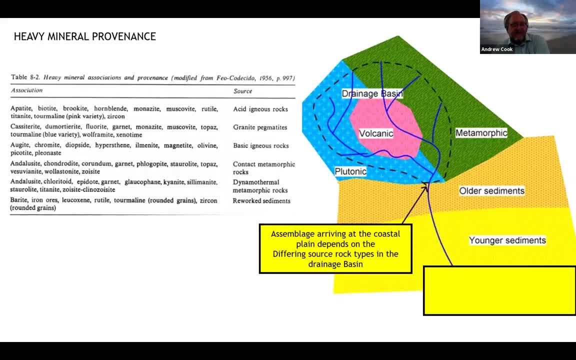 It's often associated with gneissic terrains. You can get it from the more foliitic lavas. they tend to be a bit richer Rutile in comparison. it's quite rare. it requires much more specific pressure and temperature conditions to form. 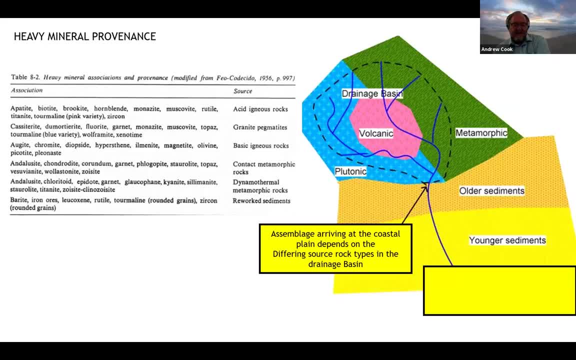 and it's likely to arise from mafic amphibolites or maybe high-grade polytic metasediments. Zircon, probably 20-fold less common than ilmenite, is more abundant in granitic terrains, particularly alkali granitic source areas. 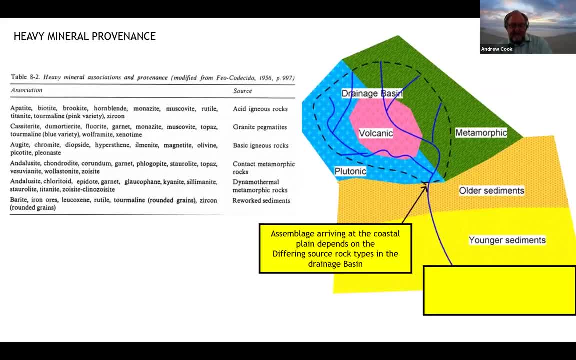 Of course I've yet to mention a small accessory mineral, usually only a percent or so of the heavy mineral assemblage, but one that's gaining increasing interest in monazite, which is a rare earth phosphate. I look at separated monazite, but mostly because it was mildly radioactive and we've sort of put it. 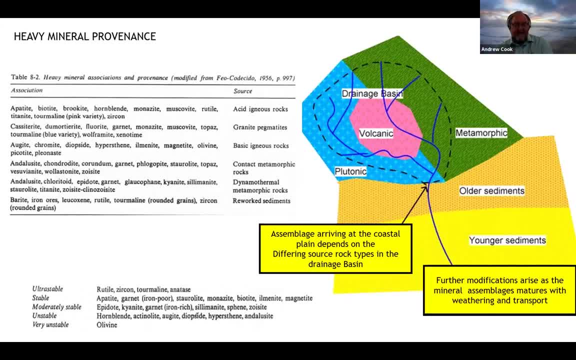 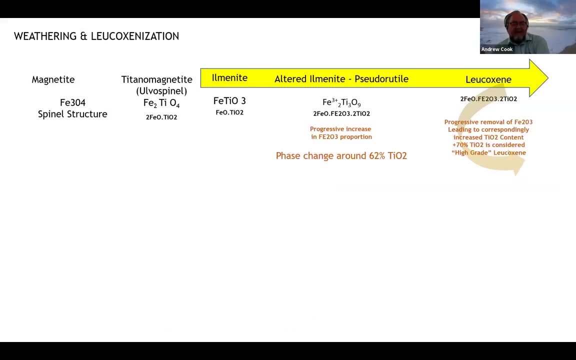 aside, and just recently we've started reopening the old stockpiles because of the burgeoning demand for electric car motor magnets and the like. So the weathering and leucoccinization of ilmenite- This is the bit I was talking about, where you could glaze over for a few minutes. 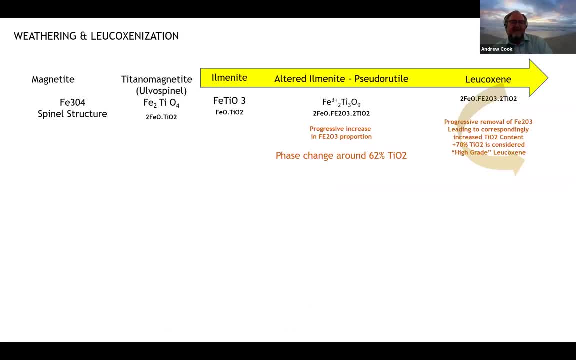 but there is a sort of continuous series of alteration from ilmenite towards leucoccin and it really in, in, in, in, in in revolves around the rusting, if you like, of the iron phase from FeO to Fe2O3.. 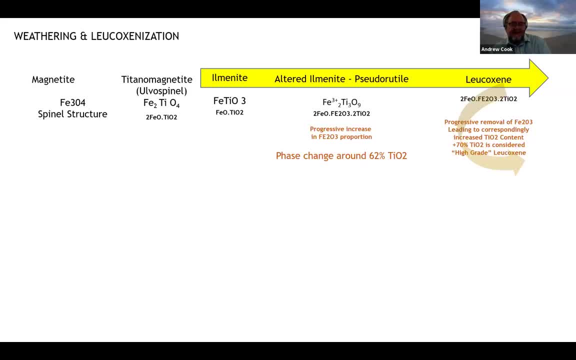 That Fe2O3 phase is a bit mobile and is able to be washed out of grains and that gives a compensatory increase in the titanium dioxide levels, And with that you get changes in the color of the minerals too: Fresh black, ilmenite, close to 50%. 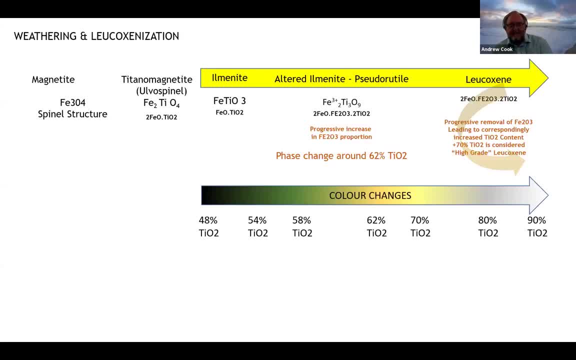 and if you look at the detergent levels you can see that they're changing color as well: TIO2. Altidulmonite perhaps becomes a bit browner, less shiny and sort of increases maybe to about 62%. Thereafter we sort of start calling it Lecoxine and there's a progressive increase. 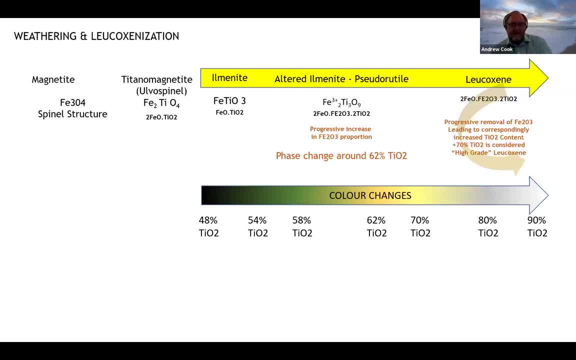 right up to around 90% or so, almost comparable with the 95% in natural rutile. And of course these different phases all have industry names and they all relate to the processes that are used for those different minerals. So you have Sulfate, Dilmonite, Chloride Dilmonite, minerals that are suitable as feedstock into 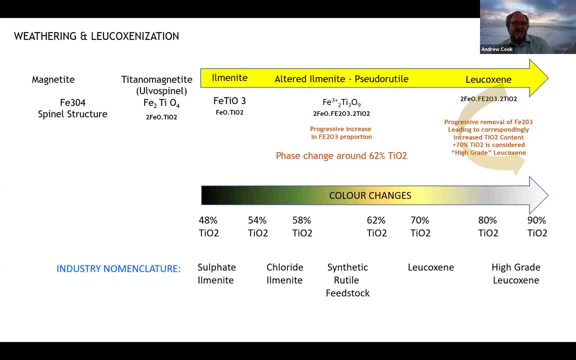 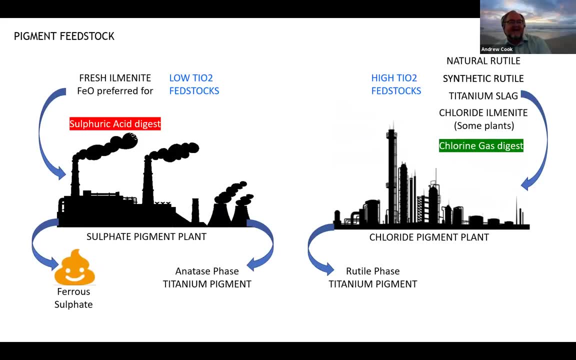 synthetic rutile plants or just sold as Lecoxine. And that leads me to talking about pigment feedstocks, because that's where our minerals go. There's two basic processes that are used to process titanium minerals, and the ultimate aim is to produce a white pigment, titanium dioxide pigment. There's the Sulfate process. 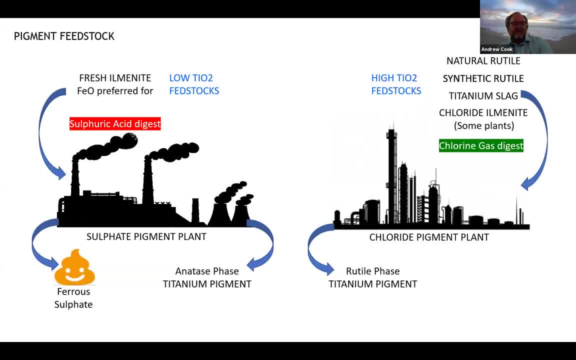 and the Chloride process. The Sulfate process uses sulfuric acid to digest basically fresh Yulmanite, low titanium Yulmanite feedstocks, not fedstocks. The process is quite simple and the plants are relatively cheap. They do have a problem in that they produce a lot of ferrous Sulfate. The Chloride plants 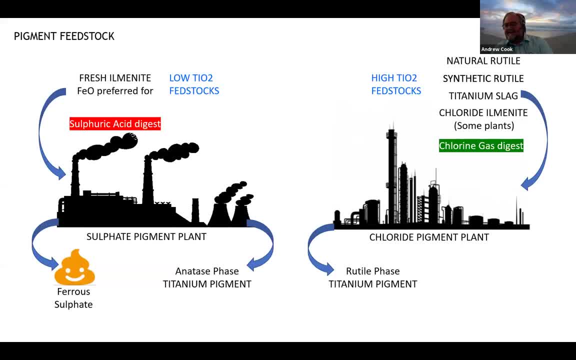 on the other hand, they're a hot gas fluid bed type process. They start with minerals that are already high in titanium, like natural rutile or synthetic rutile, or perhaps titanium slag, which I'll talk about a bit more, or, at worst, Chloride Yulmanite. These plants don't have the 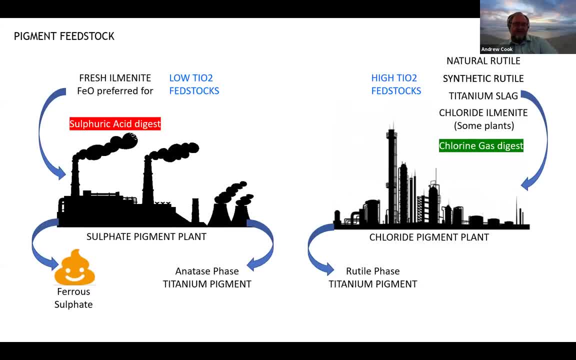 적이waste issue. so there was a bit of a trend worldwide to switch from Sulfate plants to Chloride plants as more environmentally acceptable. That was reversed for a decade or two when the Chinese entered the business. They went back to the easier and cheaper technologies and 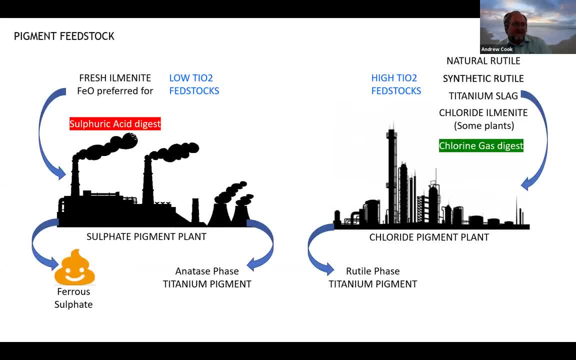 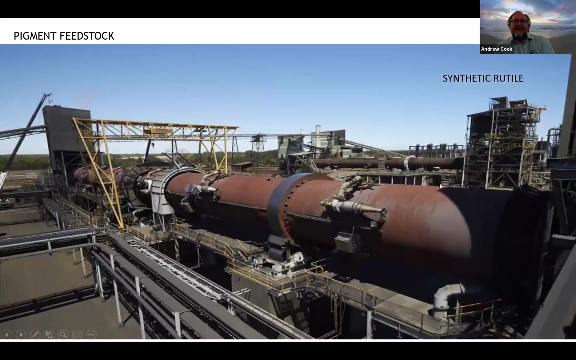 the demand for sulfate type feedstocks has increased dramatically in the last decade. it's more than, I think, 50% of the market now. But even the Chinese are environmentally aware and there is a progressive move there to switch to chloride type plants. So what you're looking at now is a synthetic rutile. 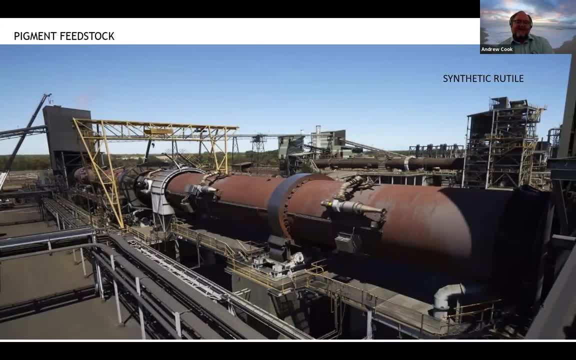 plant. This is a process that is used to convert the low-value ilmenites sort of thing that might have gone into sulfate, into suitable products for the chloride process. This one, I think, is a couple of kilns you can see there These are. 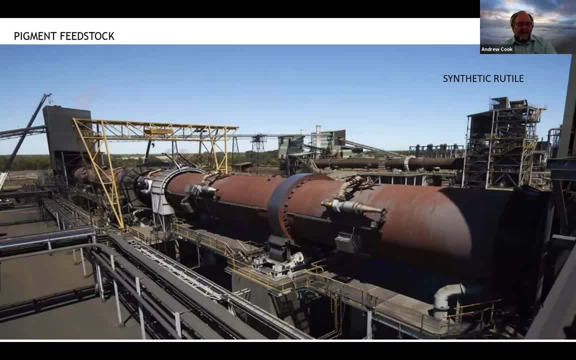 operated by LUCA down at Capel and they work by basically speeding up the look. They actually reduce the the iron in the ilmenite grains to metallic iron. then they oxidize that and rust it and wash it out to leave a sort of spongy mass which is called synthetic rutile and probably has 90 plus percent. 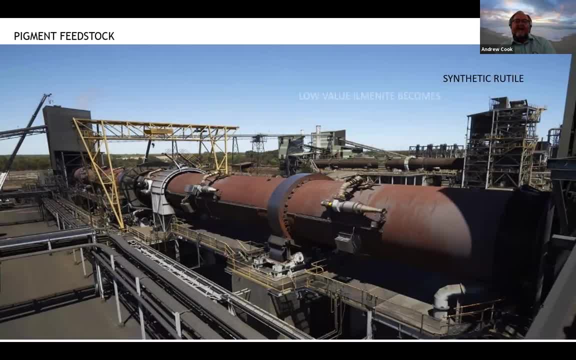 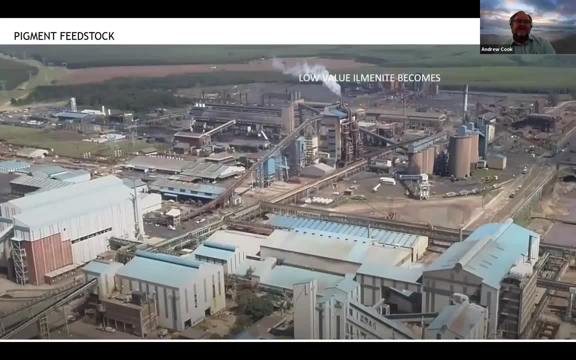 titanium in it. Another way you can go is to take your low-value ilmenite and to put it into an electric arc furnace- continuous feed electric arc furnace like this one at Richards Bay in South Africa. Your ilmenite then will be the iron will. 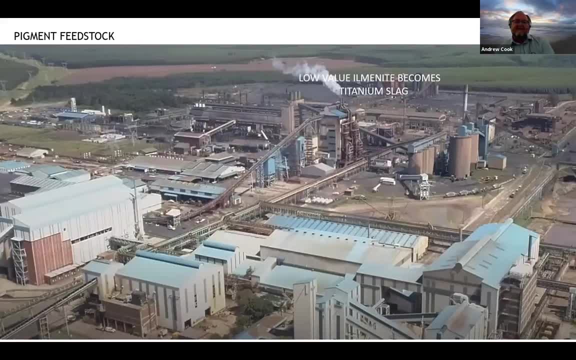 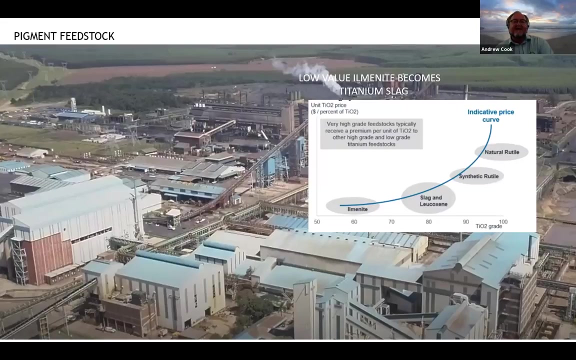 be converted into pig iron and the titanium will come off as the titanium slag, which is also a suitable feedstock into chloride plants. You probably want to have a lot of cheap electricity nearby if you're going to do one of these, But the reason for doing it is pretty apparent If you look at these: the 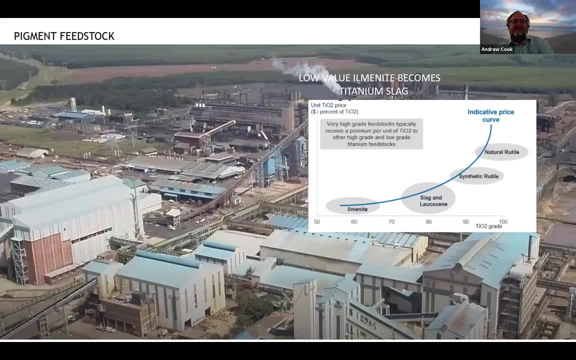 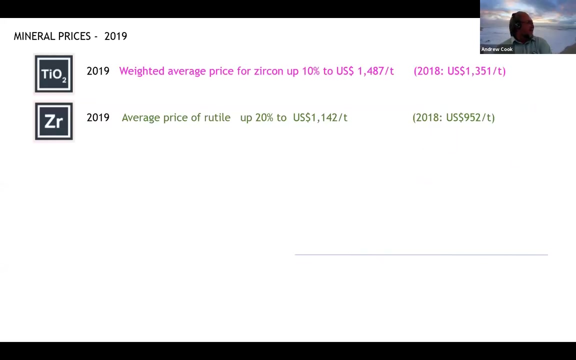 prices. relative to the TiO2 content of the different feedstocks, there's disproportionate value assigned to the higher titanium products, So that's a good way to get extra value. So we'll just talk a little bit about the prices of mineral sands. I've got some prices from last year. This year. 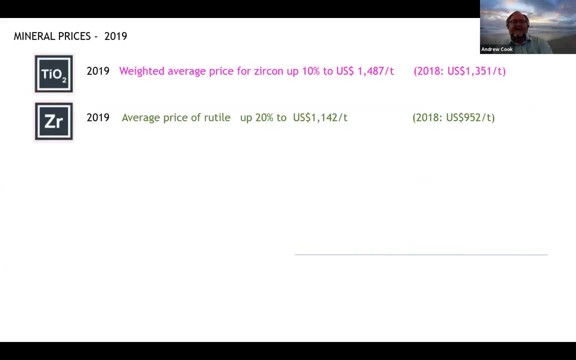 there might have been some effects from COVID affecting demand and the like, but you'll see that the average weighted price for zircon- I see I've got the symbols back the front- there- was over $1,000, well over $1,000, and for rutile. 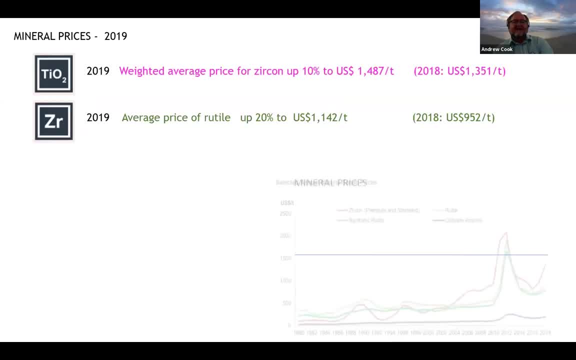 also over $1,000.. If we sort of look a bit more historically, you see that there's been a pretty steady increase in the titanium minerals over the years. Zircon is a bit more up and down and there was a sort of period of volatile gyrations around the GFC, But in recent years we sort of have moved beyond the $1,000 mark a bit. The demand for these minerals has been growing steadily over the years and no sign really of that changing as a long-term trend. You'll also get a sense from this graph of how. 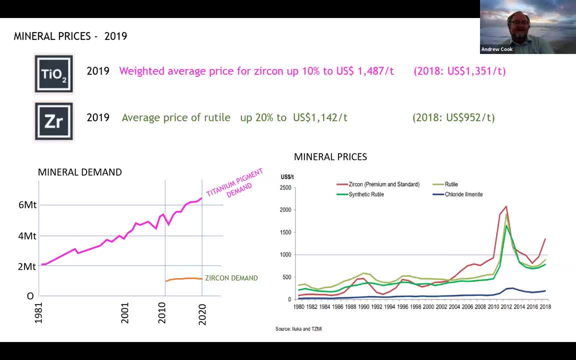 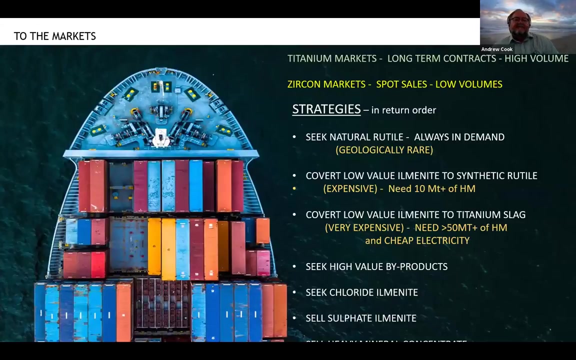 much more titanium is used for Zircon. The Zircon growth looks flat in comparison and probably only what's that? a fifth of the current volumes that you might use for titanium minerals. So you know, being larger volume things the titanium markets tend to work more with. 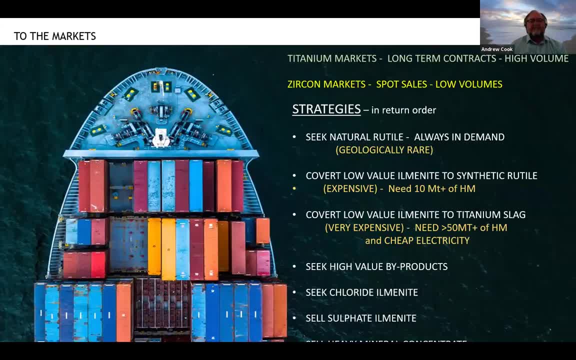 long-term contracts, Which customers will generally stick to. Zircon markets, more about low-volume, small spot sales to a large number of suppliers or customers, I suppose, And various companies will take different approaches to supplying these markets. You could seek natural rutile. 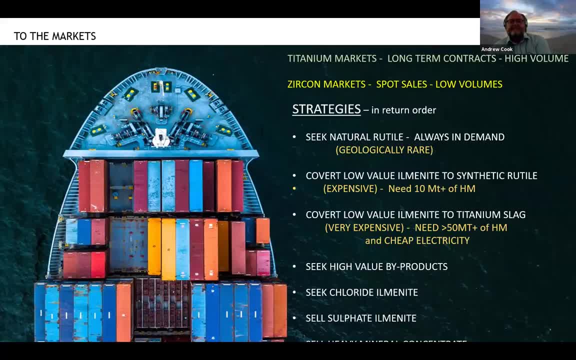 which is always in demand. And Yeah, Yeah, It's true, It's true, But geologically pretty rare. You could go the root of converting your low-value ilmenite into synthetic rutile or titanium slag. That costs you a bit of set up and 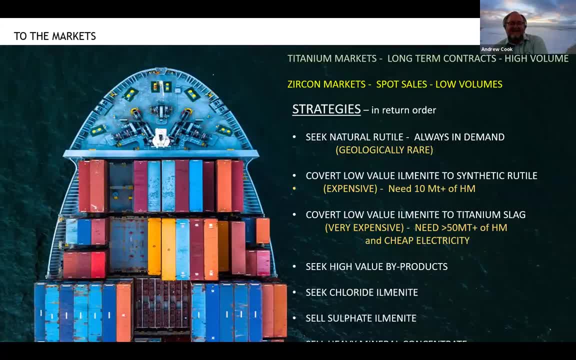 you probably need pretty big deposits to cover the cost of doing those things. Probably more than 10 or maybe even more than 50 million tonnes of real steel- Yeah, that's a good question. actually million tons for a long life payback on those plants. Another route is to focus. 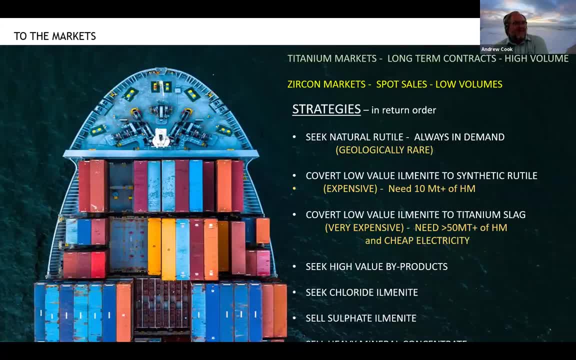 on getting the high value byproducts that go off them. with the titanium minerals You might have an ilmenite mine with high levels of rutile and zircon and that can add substantially to the value of your ore. This is the sort of route that Iluka traditionally takes. You can find chloride ilmenite, which 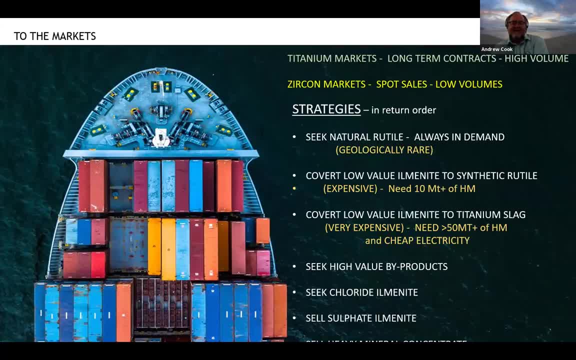 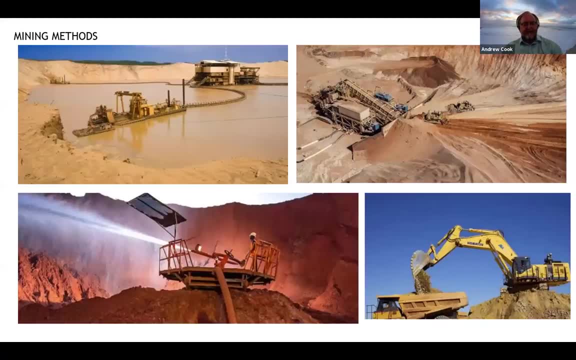 is perhaps a bit more valuable, or just basic sulfate ilmenite to sell into the Chinese market. So a bit on mining methods. There's a variety of methods used. You've got large dredges. They are suitable for loose, low clay sands and by processing maybe up to three thousand tons an hour you 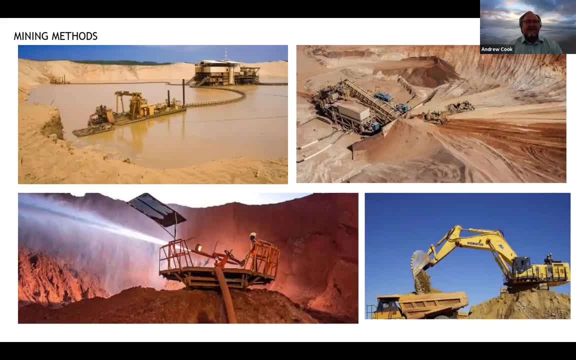 can put some very low grade deposits through these. You'll typically find them in near coastal dune sands, where you might have billions of tons of sand to process and quite large deposits- tens or even hundreds millions- of tons- of heavy minerals- within there. 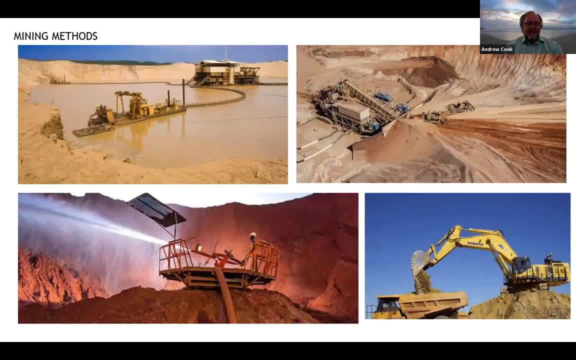 It's a bit of a long way to go. You'd be looking at sort of lower profit margins with this sort of thing, but you can have very long- mine lives and you can progressively scale up your operations and of course you'll be a long-term, consistent and reliable. 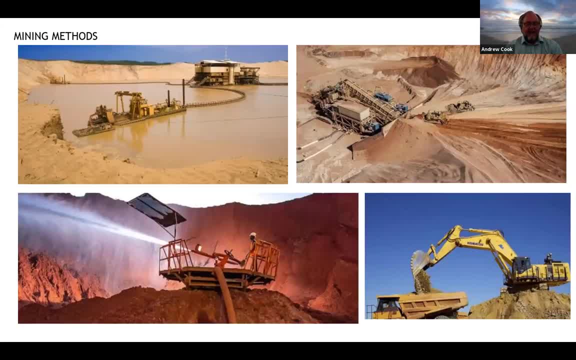 supplier to the markets. Of course, dredging isn't always applicable. It becomes more complicated if your sands are very clay and particularly difficult if they're cemented to any degree. Higher grade deposits well can be mined by more conventional truck and shovel type techniques. Iluca does this. We've progressed more these days to a dozer push type. 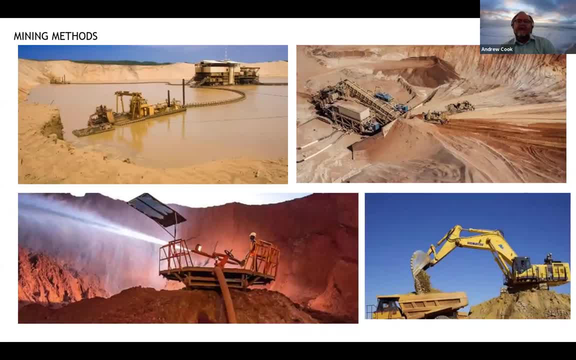 setting where you're pushing sand down into in-pit mining units that slurry them up and pump them on. You can also see a picture there of hydraulic mining. This works very well on dunal sand deposits that have a lot of clay through them, Sort of thing that's done by base resources. I think that picture is from. 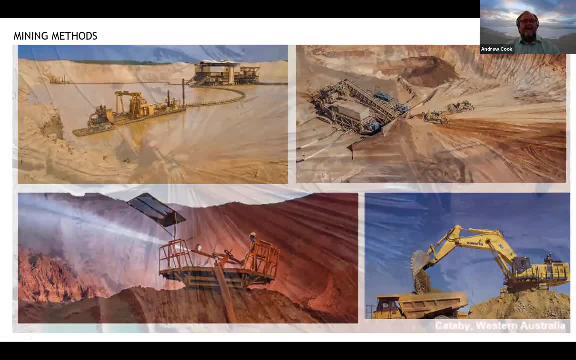 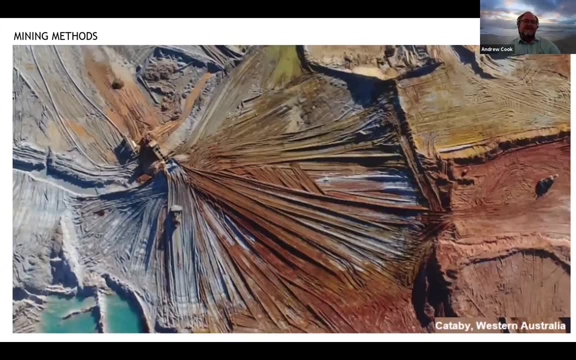 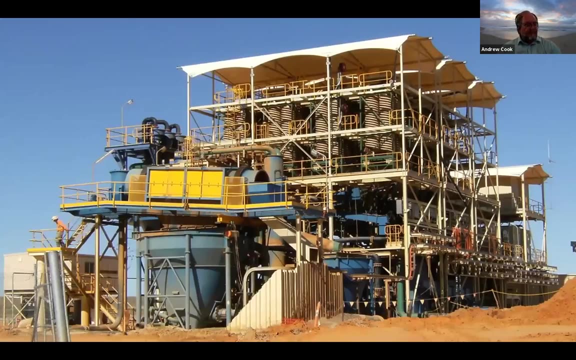 there in Kenya, And there's a shot of Iluka's new mine at Kadabi with the dozer push feeding ore down into the mining unit there. So moving on to the sort of plants that would process the oil. So moving on to the sort of plants that would process the oil. So moving on to the sort of plants that would process the oil. 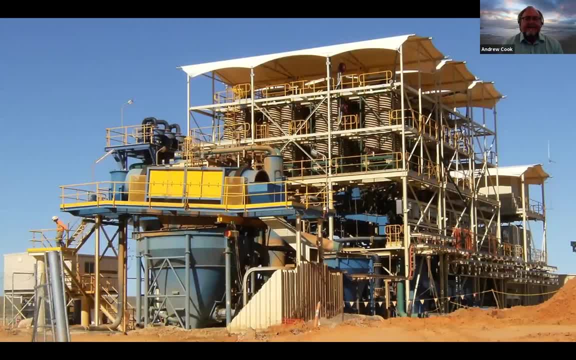 This is a picture of a what's called a wet plant from. I think this is the one at Mindery in South Australia that Australian Zircon operated. It's a nice little modular unit, was able to be pulled apart and shipped across to Western Australia where I think it's now producing heavy mineral for image. 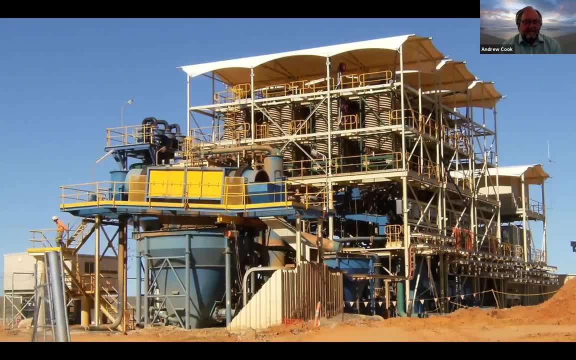 resources at Boonanaring. The ore that goes to these plants is screened of coarse pieces, usually, you know, in durated clumps of rock, And then a slurry is pumped towards the wet plant. Hydrocyclones will be used to pull the. 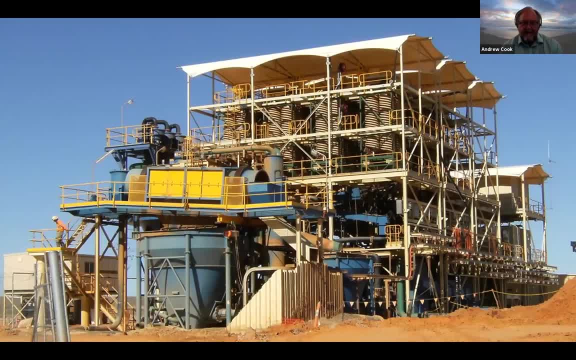 clays away from from the slurry And they are sent out to settle, usually with the addition of some flocculent chemical, And what you will then do is produce a constant density bed of sand and mineral that will pass down a series of spirals and use the centrifugal force to move. 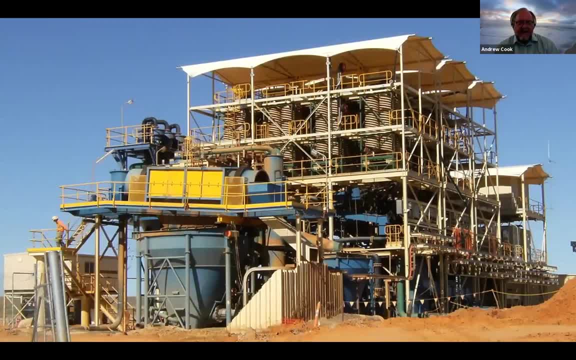 the less dense sand away from the heavy minerals And using several passes in spirals of different profiles and flow rates and with recirculating loads, you can recover as much heavy mineral as you can from the sands And it's quite common to get 80-90% recovery. The wash sands are 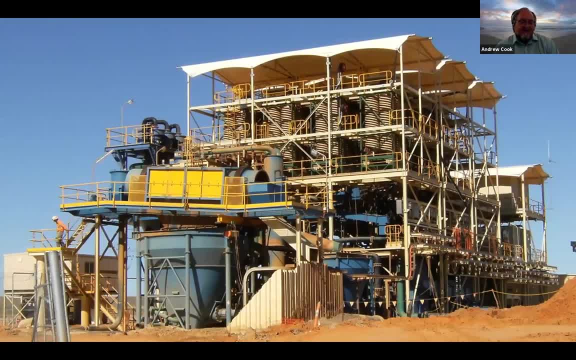 disposed back into the mining void, often co-disposed with the slimes, the clays, that was washed out from the hydro sizer. These plants will sit near the mine and they're usually designed to be shifted periodically: One, two, three. 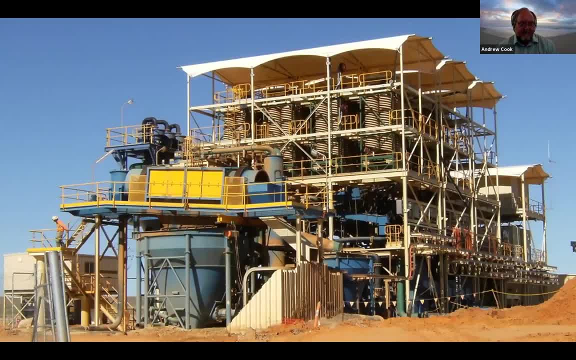 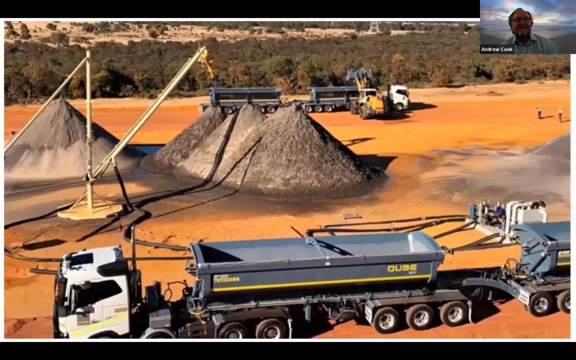 seldom more moves over the life of the mine, Or they can move on to the next deposit, like this one did. The ultimate output, of course, is your heavy mineral concentrate, And you want to take this then either to port for sale or, more commonly, to a dry plant. 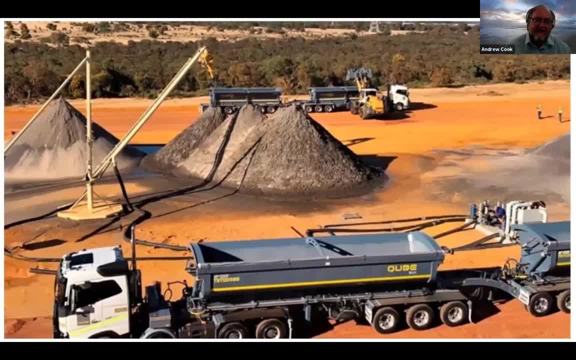 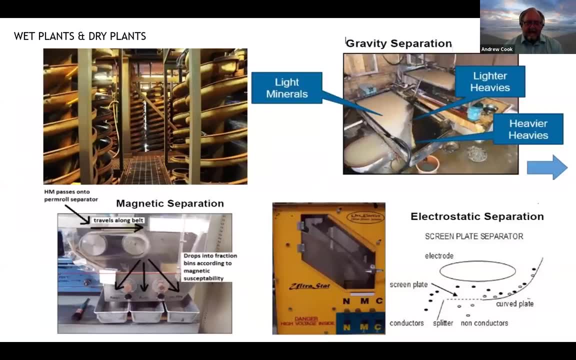 which is where you will work to separate the individual minerals. I'm showing bench scale equipment here: Magnetic separators of various styles, Using either permanent or electromagnets to remove their iron-bearing minerals, chiefly the ilmenite, And of course, as ilmenite weathers, it becomes less. 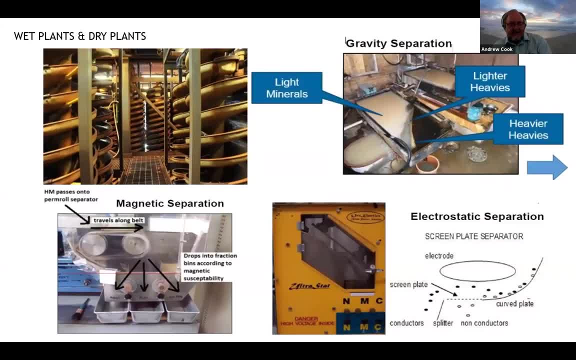 magnetic, So it's possible to progressively separate several different titanium phases using magnetic fields of different strengths. The most magnetic material termed the primary ilmenite might be the stuff that goes to sulfate plants, Or you could turn it into titanium slag and pig iron, Or you could turn it into titanium slag and pig iron. 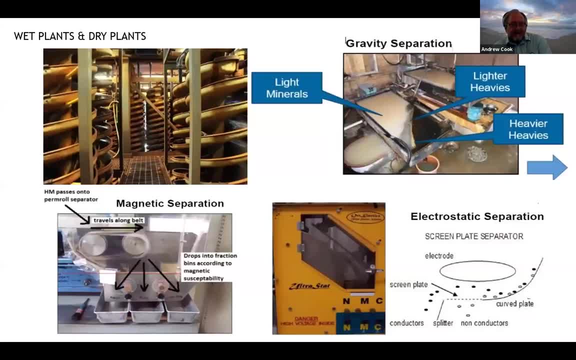 In your arc furnace, The less magnetic material needs stronger magnetic fields to pull it away And it will have a higher titanium content. So this is called secondary ilmenite. This is the sort of thing that you might feed into a synthetic rutile plant Or sell it as chloride ilmenite to 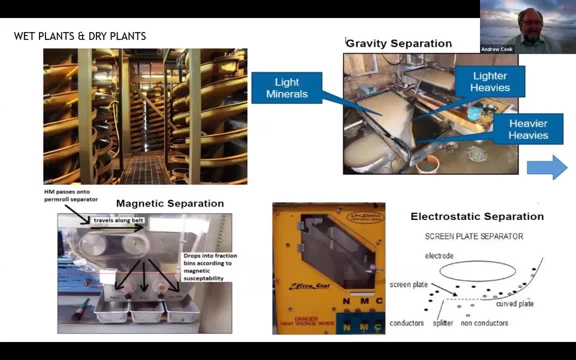 a suitably equipped pigment producer. The non-magnetic phases that pass the magnets without effect, that'll host your more valuable constituents, Your leucoxenes and rutiles and zircon, As well as a lot of troublesome aluminosilicates, Things like kyanite- that can be difficult to remove. 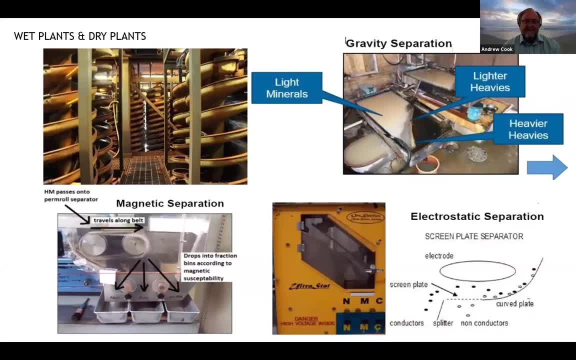 Fortunately, rutile is slightly conductive, So it will dissipate an applied electric charge, Whilst zircon, for instance, retains charge. So you can use charge attraction and repulsion To direct these minerals away from one another And so separate rutile and zircon products. 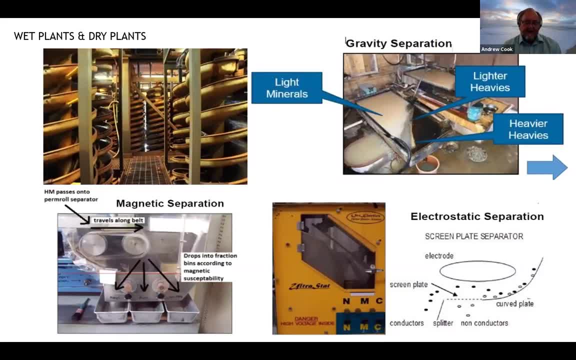 Both wet plants and dry plants work best when the feed is fairly consistent, Because there's a lot of tuning required to make these plants work effectively. So mineral sand plants tend to be quite metallurgist, heavy. And of course, even when you separate the minerals, there's further considerations that affect the 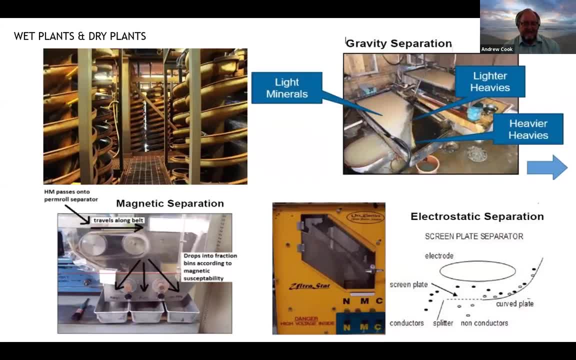 marketing of those minerals Specifications to be met. Different levels of contaminants You might have, say chromium or niobium, affecting your ilmenite. Customers don't like that. Iron, uranium and thorium levels in zircon have to be monitored. 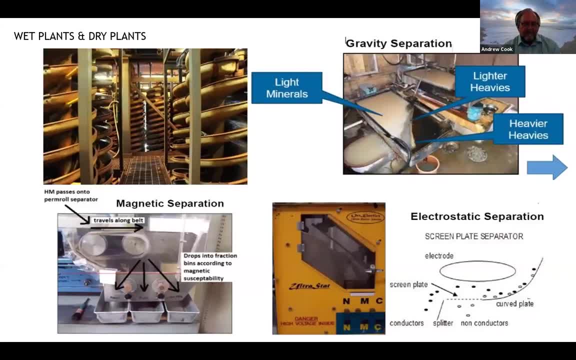 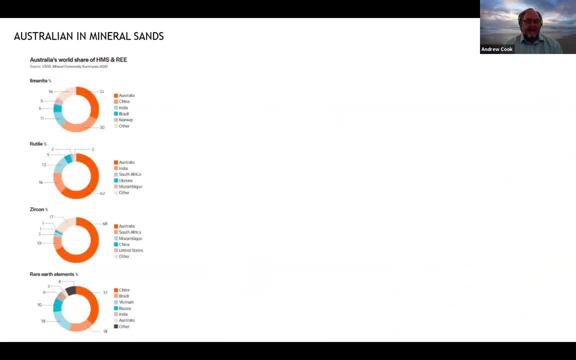 So you have to be careful A little bit about Australia's role in the mineral sands industry. Here's a graph of some pies showing where we are with the different minerals, Australia being in the brown there, And so you can see we're quite a dominant player in the mineral sands industry. 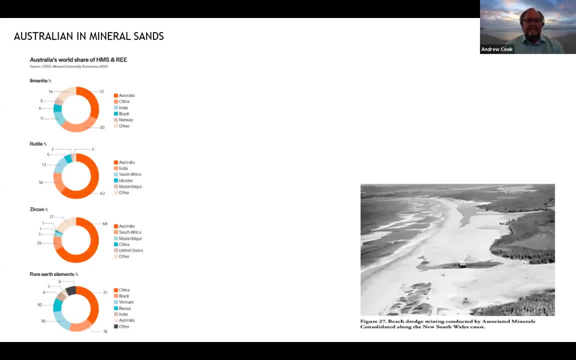 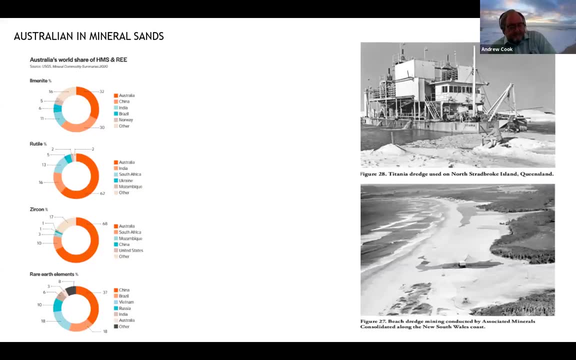 And in fact we were one of the first countries to seriously get into mineral sands. We had post-war immigrants like Joe Pinter, who experimented with separation equipment in his backyard in Melbourne, Finding ways to separate rutile and zircon, And that, you know, allowed a. 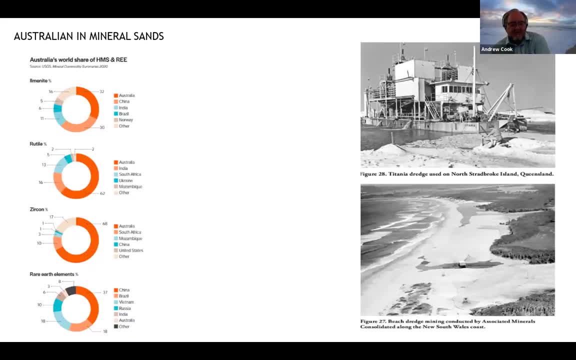 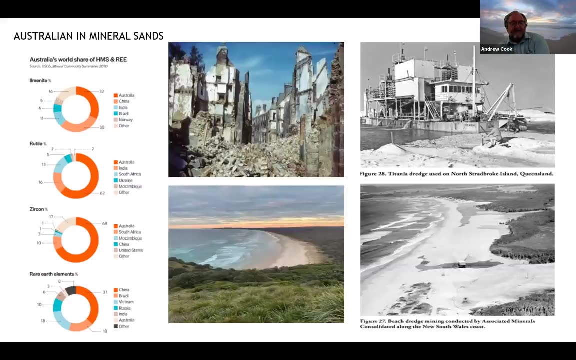 ragtag bunch of small sand miners from the beaches of northern New South Wales to eventually be consolidated, mostly by British mining houses, into an industry that came to dominate worldwide. I'd guess finding yourself working in the beaches of Byron Bay must have felt like heaven after fleeing war-torn Europe. 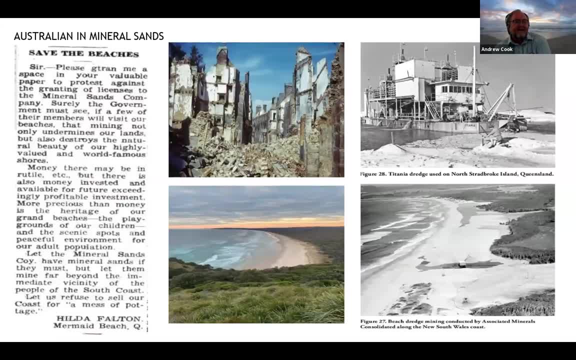 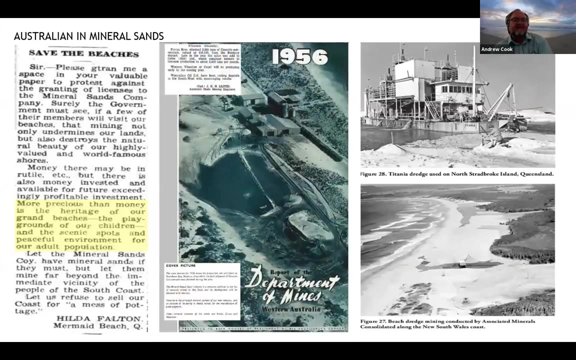 But eventually you had a closure of the mineral sands operations on the east coast, People like Hilda Felton here writing in about why our precious beaches were being despoiled And that actually led to a shift in the industry more towards Western Australia. 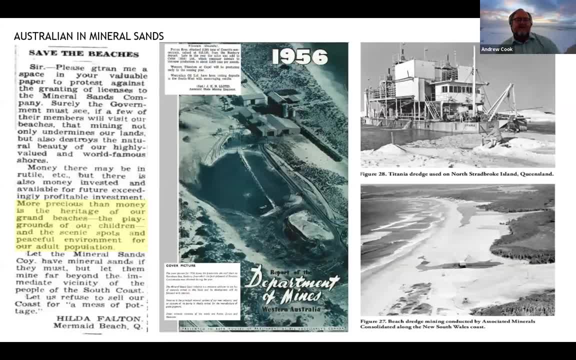 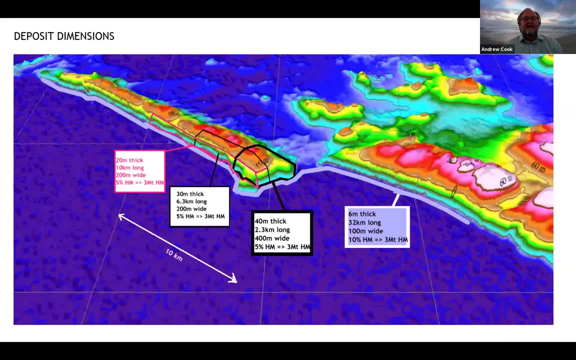 There's the first report of the new industry opening in 1956 down in Bunbury. So a little bit about the dimensions of mineral sand ore bodies. The ore body dimensions required to host enough heavy mineral for an acceptable positive return on the establishment costs of a mine are surprisingly large. This example shows the 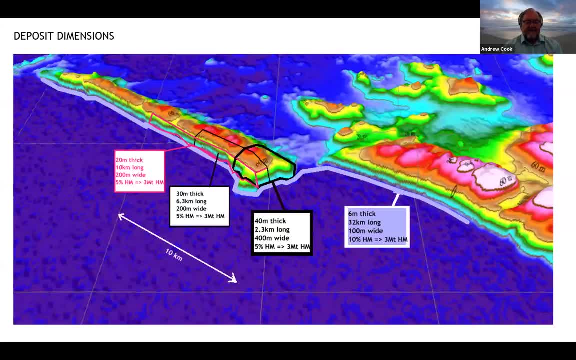 dimensions that you might need to generate just three million tons of contained heavy mineral at five percent average ore grades. You could have thick, broad dune deposits, maybe five to ten kilometres in length, or narrow beach places Where you might need tens of kilometres in length to generate three million tons of heavy mineral. 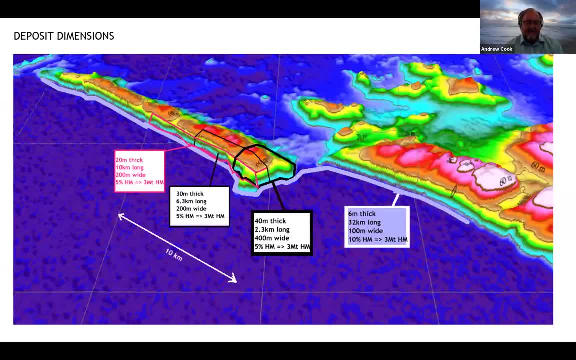 The practicality of this is that strandline or beach deposits won't usually be sufficient on their own. It's more common for a mining area to host a number of beach deposits formed at different times in close proximity- Camper deposits, if you like- formed where long-lived. processes have have acted locally And just you know, to set up a mineral sand mining operations cost you something somewhere between 100 and 400 million dollars. So to get a reasonable return on investments of that scale, you probably don't want to look at things much smaller than about two million tons of contained heavy mineral. 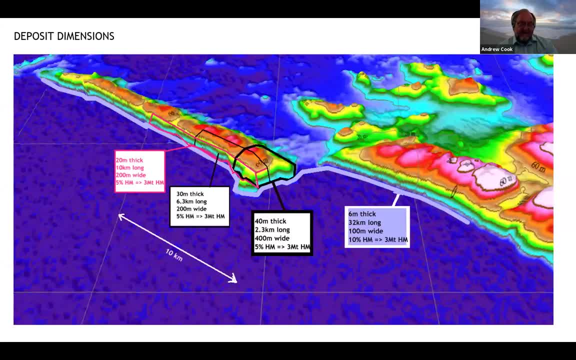 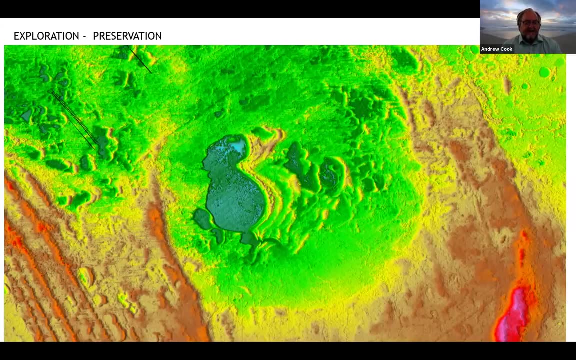 If you've got low ore values, you're probably going to need even more, maybe 10 million tons of heavy mineral. So we'll look a little bit now at the facets of exploration. So when we're looking for these deposits, it's not so much the modern beaches- 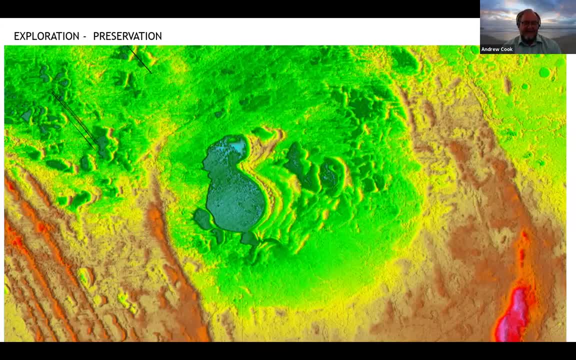 They're somewhat sacrosanct. People don't like seeing them disturbed or defiled. We're more looking for ancient beaches, Beaches that have been stranded inland by recent or tertiary aged sea level changes, or beach deposits in older sedimentary basins that the sea departed. 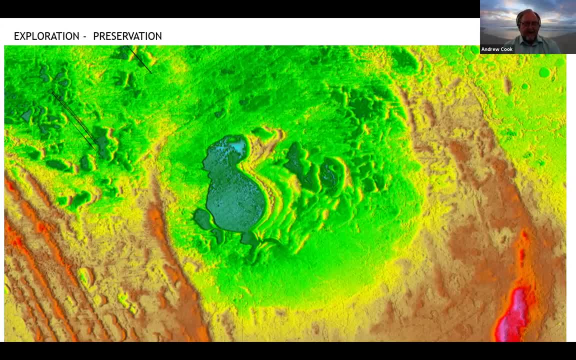 long ago. Here's a digital terrain model from the Murray basin, with some well-preserved beach ridges in the bottom left. there You'll also see a lake bed once larger And a tectonic ridge on the bottom right, all with windblown sand overlay. 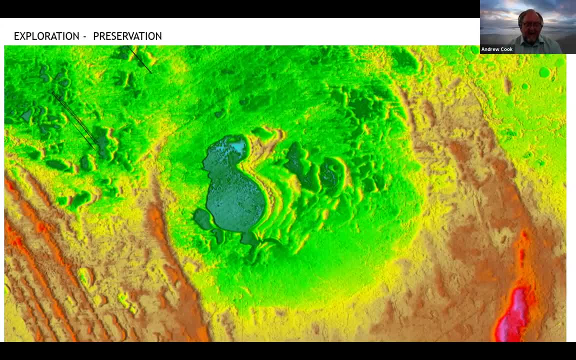 The deposit setting those fine white black lines towards the top left. there that's the WRP deposits that were mined by Aluka And you can see there's not much sort of geomorphic indication that they're there. So terrain models are a very useful start, but you often have to look a bit further than that. 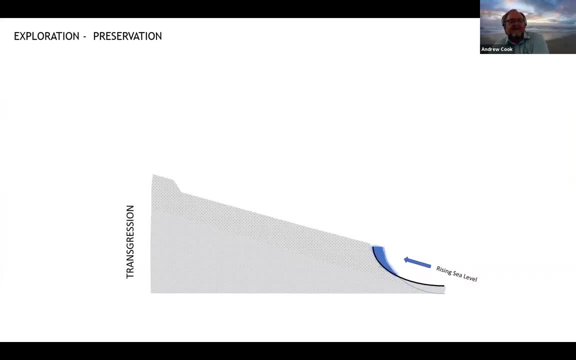 So, talking about suitable environments for the formation of heavy mineral deposits Where sea levels are rising, well, rising and falling sea levels really are the drivers of deposit creation. When you get a rising sea level like this, you'll tend to see that the beach is being eroded and sort of deposited out the back and as the sea level rises, 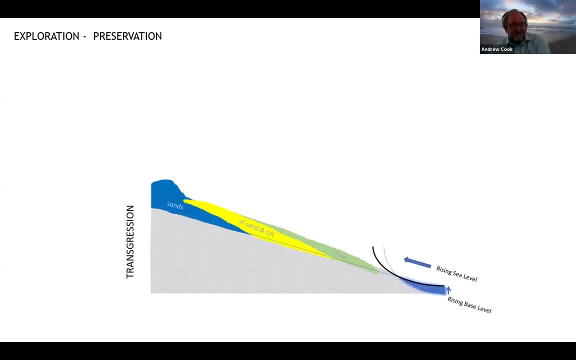 you'll end up with a situation like this: Thin deposits of well-sorted but only weakly mineralized sand. These seldom have commercial grades And a lot of you know a lot of smoke in these, but you know not much fire. You can waste a lot. 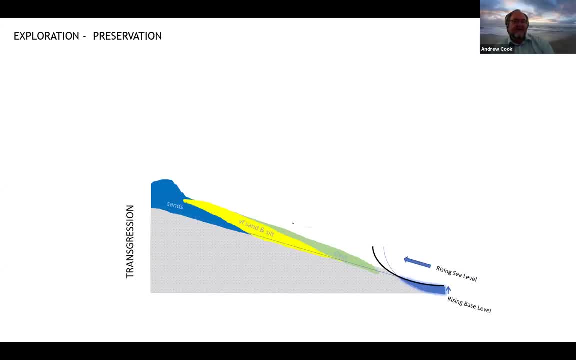 of time looking at this sort of thing. The place you really want to go is in the regressive phase, where the sea is, sea level is falling and the land is building out. Deposits formed here obviously have a better chance of preservation And also sea level leads to reinvigoration of the drainages. sea level falls, reinvigoration of 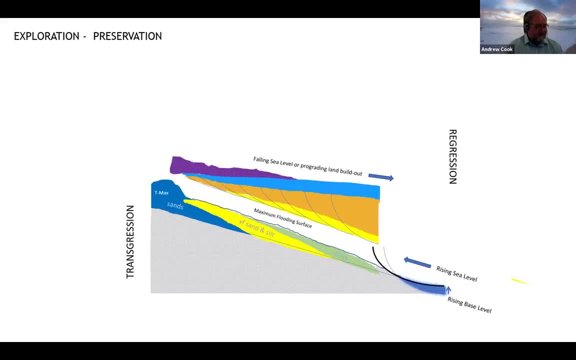 the drainages behind, so that delta sands are now washed down to new base levels and you have increased sediment supply of sand to the coast. The transition point between transgression and regression, termed Tmax, is a very good place to look. You can see that there's a lot of sediment. 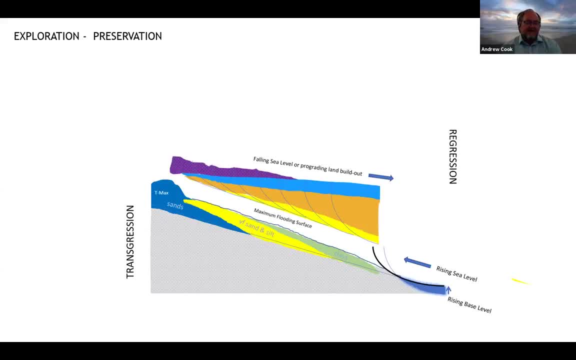 there. This transition can be slow, so the beach position can be present there for quite some time. You'll also find that very often the escarpment that was cut by the transgressing sea is still preserved, And the Witcher and Gingin scarps and the Perth Basin are classic examples of this. 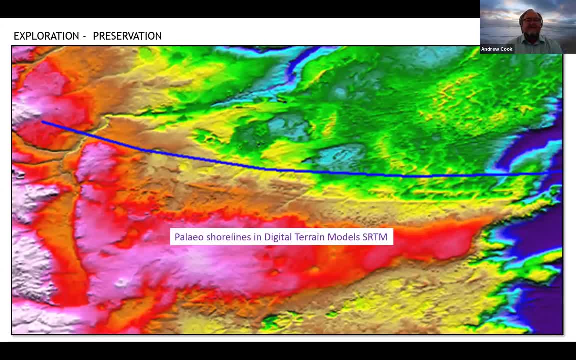 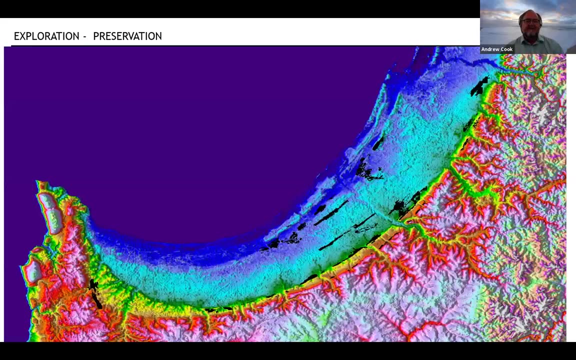 Here, for instance, is a picture of some strained ridges in the terrain model that were left by regressing shorelines. This is some of the ones that we explored recently in Kazakhstan, And here's a picture of that scarp I was talking about in Geograph Bay, the 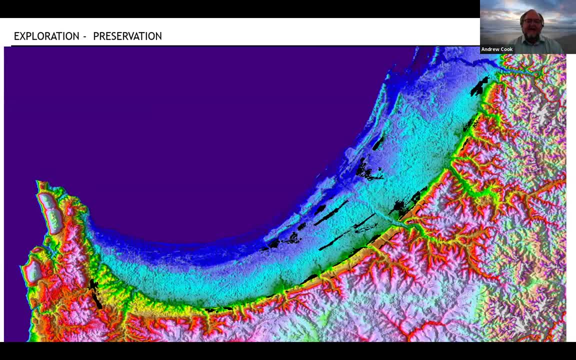 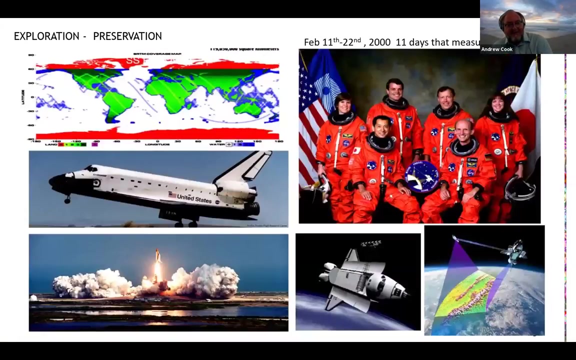 Witcher scarp. You can see the black outlines of a whole bunch of mined mineral sand deposits Developed there and obviously a real focus at the back against the scarp in the Tmax position. A bit of a shout out while I'm doing what, I'm talking about these things to the 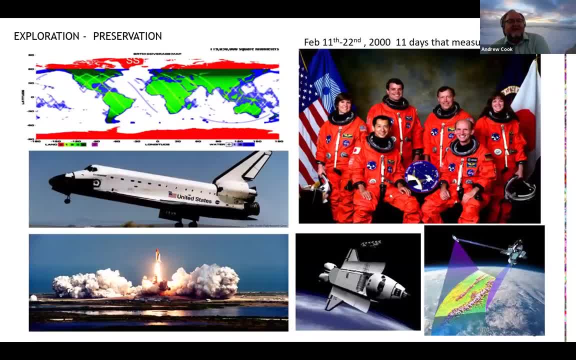 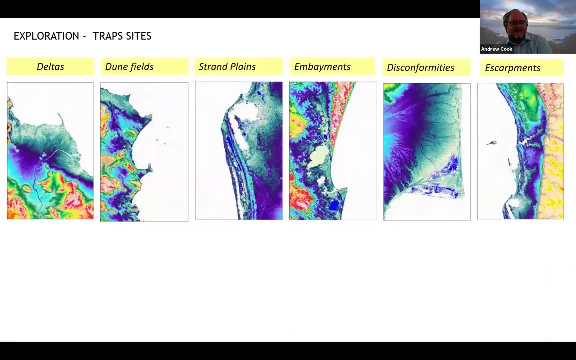 the SRTM shuttle digital terrain model data all collected in the space of 11 days in 2000.. This has become a real tool of the exploration of the Tmax. This is a really good example of the explorer these days, And here's an example of a whole bunch of depositional environments. 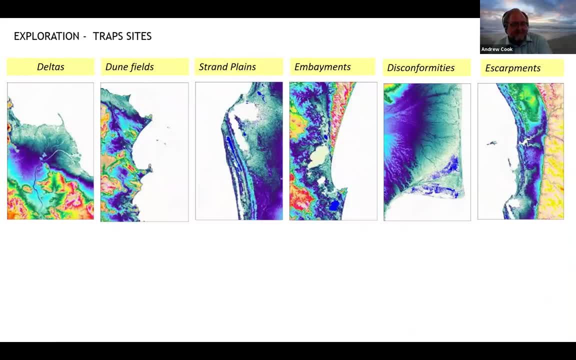 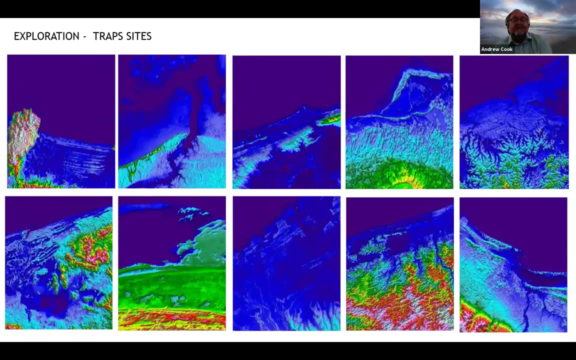 shown as digital terrain models that I've flung onto the page here. Storms in winter. We should move on to show you some more there. All these are settings that would catch the eye of the Mineral Sand Explorer. You can see some strand planes there. 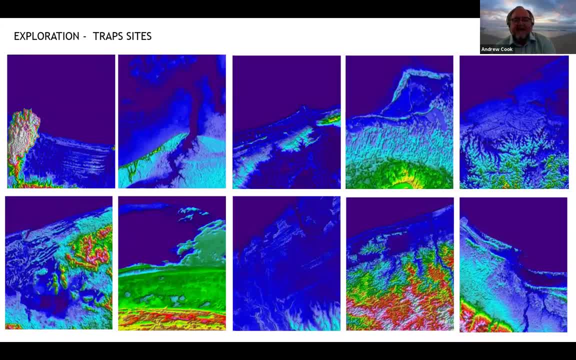 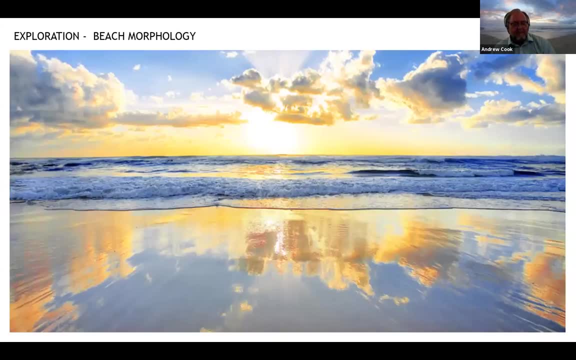 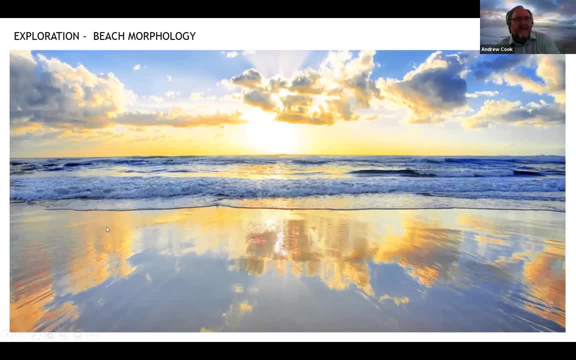 I'll skip ahead a little bit here. I'll skip ahead a bit because I think we're running behind and talk about beach morphology When you hear me talk about reflective beaches in a minute or two. this is not what I mean, But it does show that we have nice workplaces as Mineral Sand Geologists. 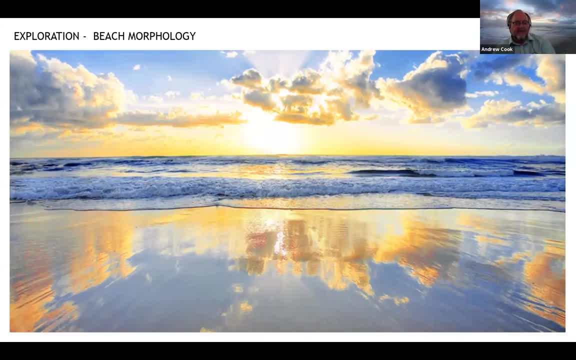 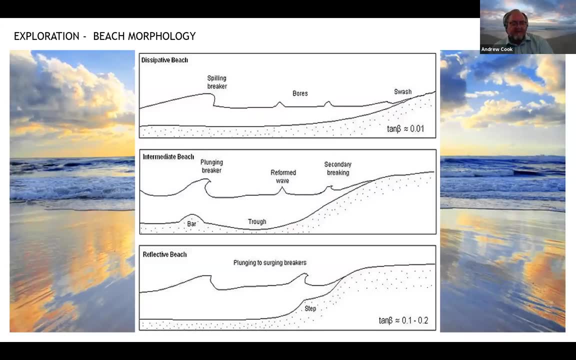 And you can think about this picture when you're logging your iron colours up in the Pilbara. So wave energy affects the deposition of heavy minerals. It also affects the morphology of the beaches. Beach morphology in turn determines the capacity for the beach to generate and. 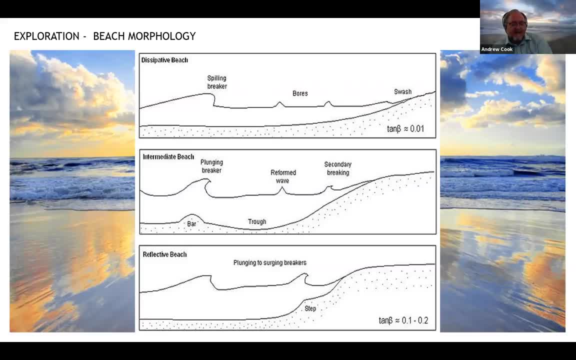 accumulate concentrations of heavy minerals. Steep beach profiles with reflective waves- the example shown at the bottom here- are usually narrow. They have good capacity for periodic erosion, and that in turn captures heavy mineral concentrations. They can be maybe six to eight metres tall. 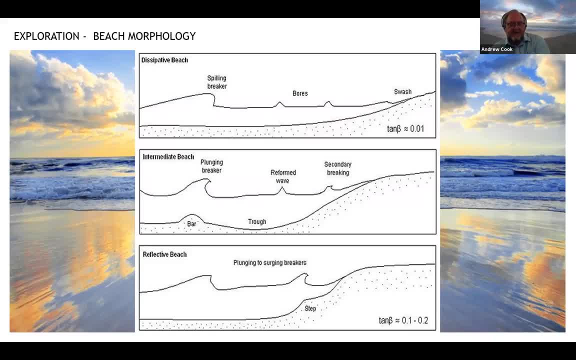 Shallower beach profiles, where waves shoal across broad zones before impacting on lower energy. swashstones are dissipating for the energy of the waves, So they have less capacity for beach erosion. Deposits that form there are thinner. Maybe your beach package might be only two to. 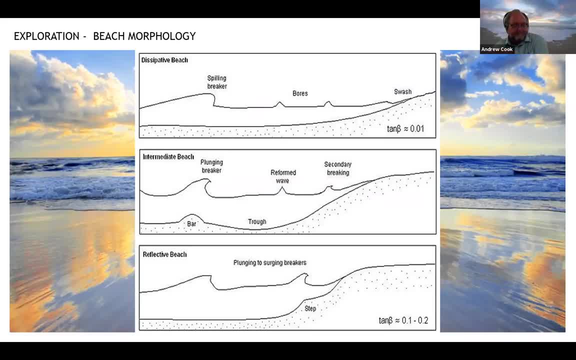 four metres thick in that upper case, And I should mention, though, that nearshore shoal sands can be quite broad, in this case in the dissipative beach, and if seasonal storms are regular, then the deeper probing waves during the storms can actually winnow the sea floor to a degree. 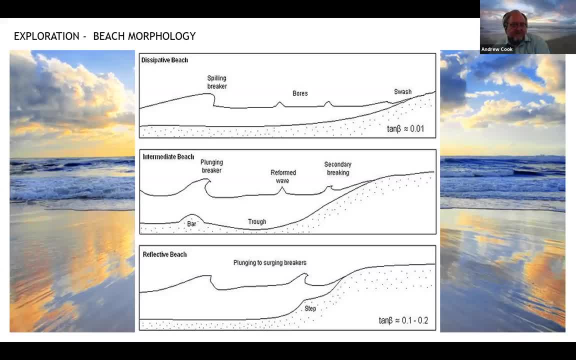 creating distinctive hummocky cross stratification. ripples and heavy minerals can accumulate in these. The grades don't normally achieve the levels possible on the beach, but the volume of material in the shoal banks can exceed if the frequency of the的話. saint was magari 적otăm 가. 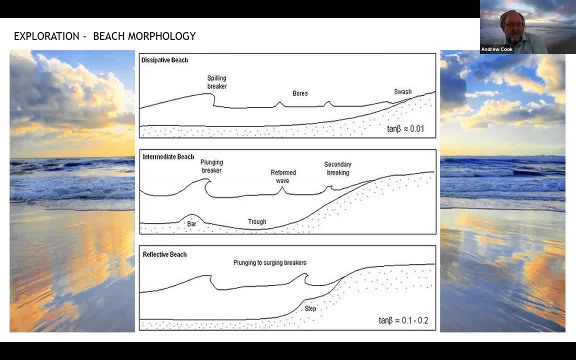 пов 산ningen exceed the onshore beach environment by an order of magnitude. So there are deposits formed in this setting, the style we call WIM deposits. They tend to be finer grained. There's some large examples in the southern Murray Basin and the Gippsland. 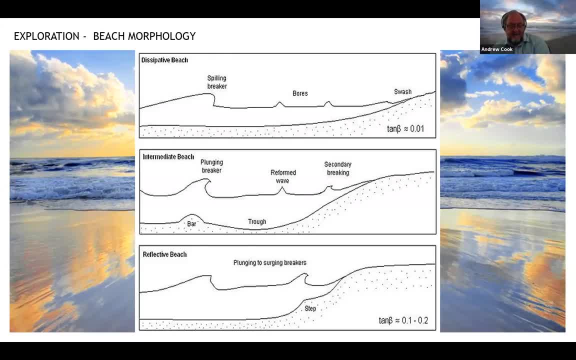 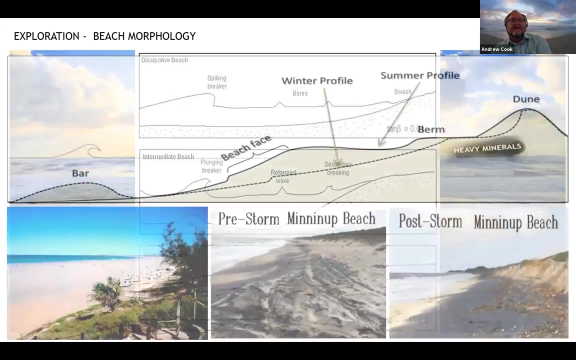 region of Victoria and Oluka is looking into these as new development options. Tides is also worth a mention. The effect of tides is not good. A greater tidal range will smear out the beach over a broad zone, I think Cable Beach up in Broome there on the left. 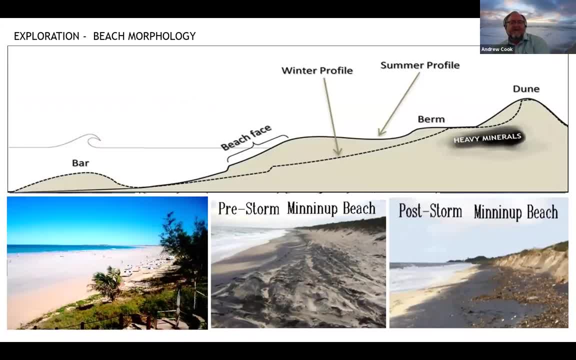 whereas you can see an example of a steeper more reflective beach here at Mindenup down in the southwest of WIM. This one actually has a lot of heavy minerals on it. The other point that's worth mentioning here is the effect of 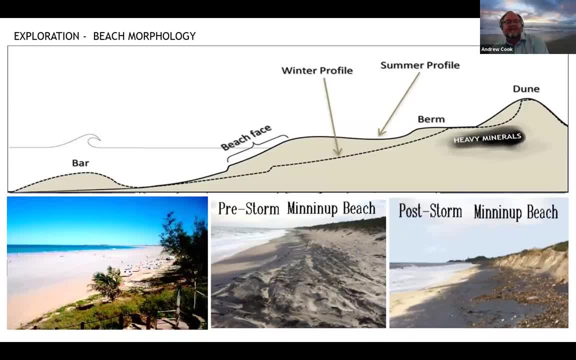 climatic or seasonal changes. Most beaches will have a sort of summer and winter profile. The storms of winter will move the sand offshore and quite often the heavy minerals that are in the sand can be left on the back beach as a concentration there. This will later get buried as the 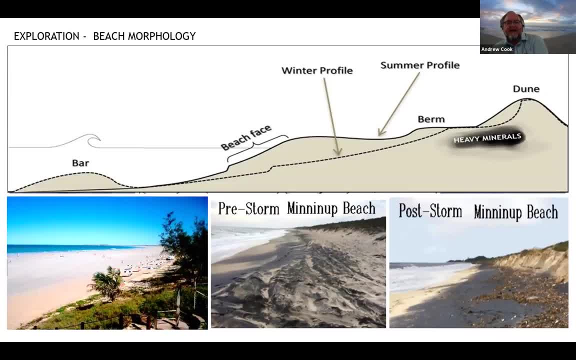 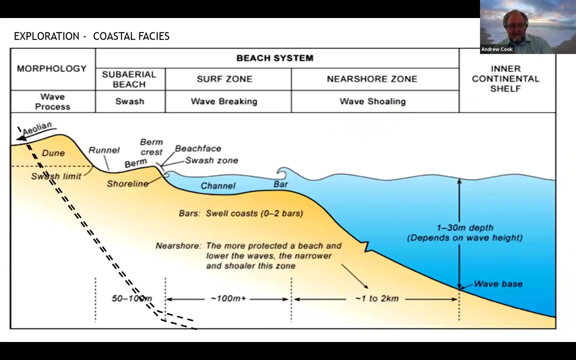 normal profile, the summer profile returns and that is the basic formation process of beachplacer deposits. The pictures in the bottom there show Mindenup post storm and pre-storm and you can see things are much blacker post storm. You can see that there's a lot of sediment in the sand and there's a lot of. 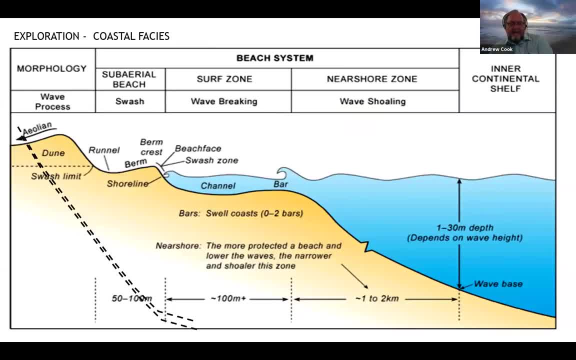 sediment in the sand. So how do we spot a prospective beach horizon, which might be only two to four meters thick, when we're looking at a big body of regressive strand plane sediment? The way to do it is to look for the different facies that are generated on the beach. 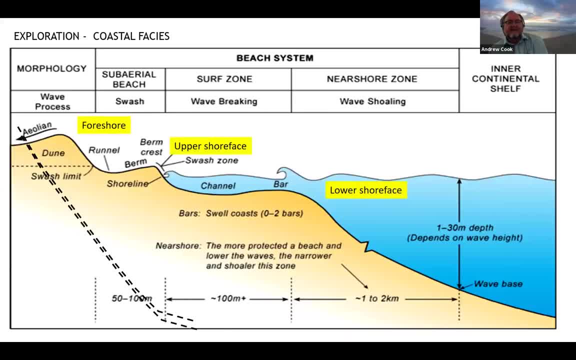 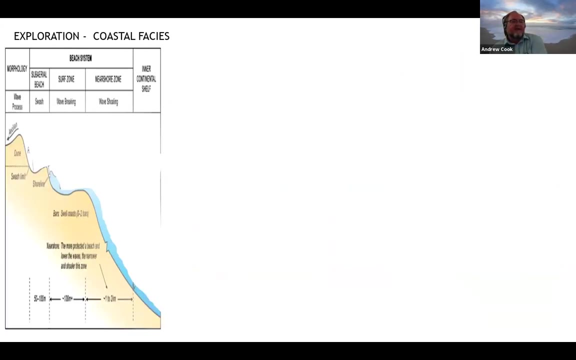 Here is one. Here is the classic beach profile picture: Lower shore face sands deposited underwater and upper shore face the beach at the interface and then the foreshore where those heavy minerals are deposited on the back beach and and the dunes. If I compress that up for a second and we look at the pattern of 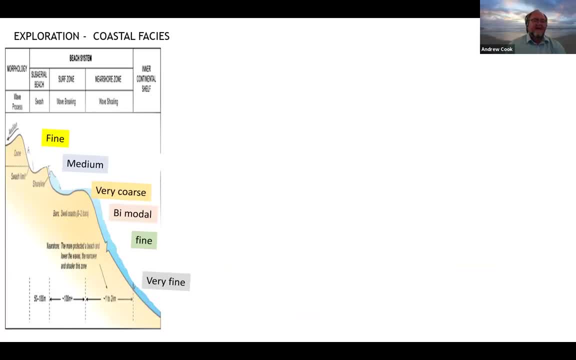 grain sizes that occurred. you'll see that there's a pretty distinctive finding as you go offshore: Quite a coarse or very coarse zone, maybe even pebbly or granules, where the surf is crashing on the offshore bars. Beaches more typically be a medium sand and the stuff that blows up into the 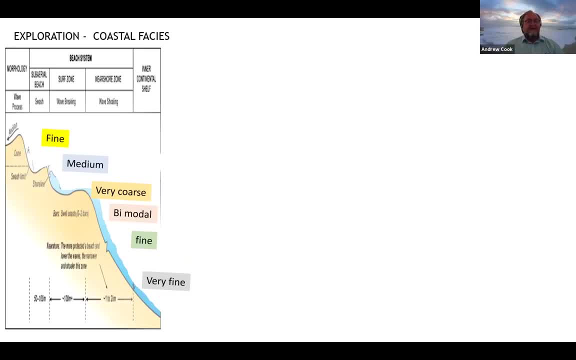 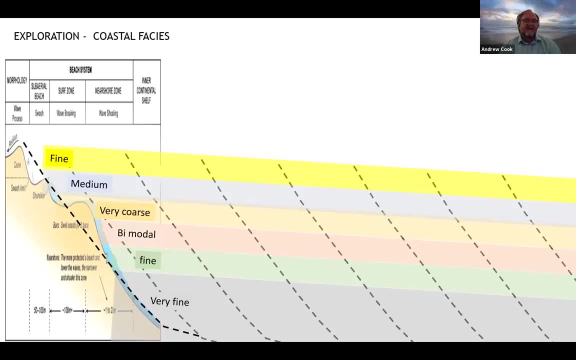 dunes is fine sand. And if you take that pattern and you have the land building out progressively for a series of beach positions, you end up with a sort of layer cake pattern of varying grain sizes like this And the expected beach position or the beach position itself is a 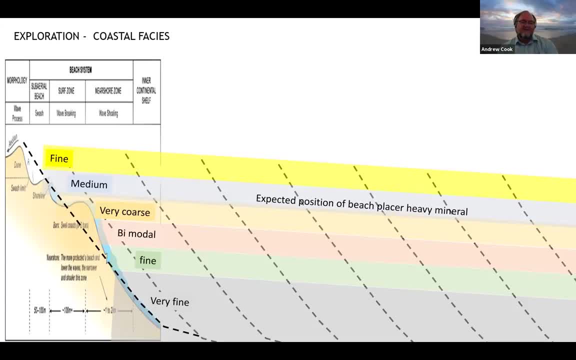 a flat layer there that's readily identifiable, most easily by the fact that you have the very coarse sand layer under underneath. So when you're drilling down through these sands, you're looking for this pattern that's guiding you to where the beaches, where the heavy minerals might be expected. 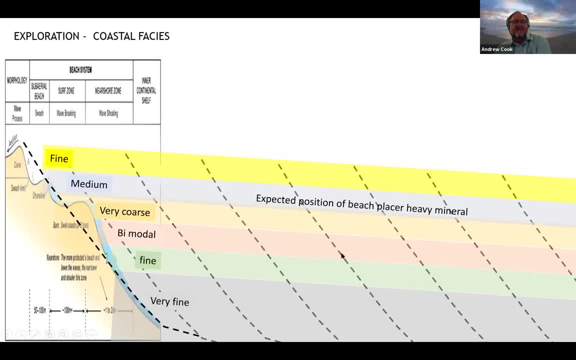 The shoal deposits I mentioned before will be down here in the just offshore positions. So ILUCA assembles all this information and we use it to generate a lot of sand. So ILUCA assembles all this information and we use it to generate a lot of sand. 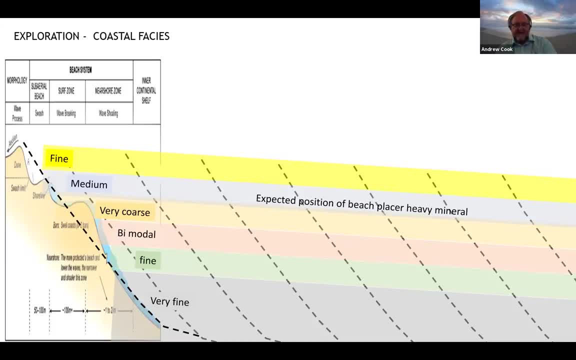 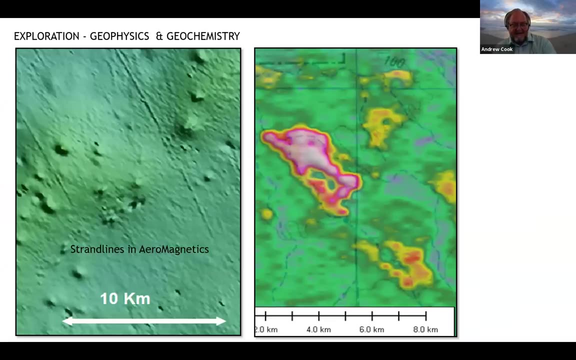 We can also generate global prospectivity models. we can decide where to look. These are being continually refined and updated. I'm not going to show you them here, but there is always, you know, real world overlays to consider after that whether it's practical to access or gain. 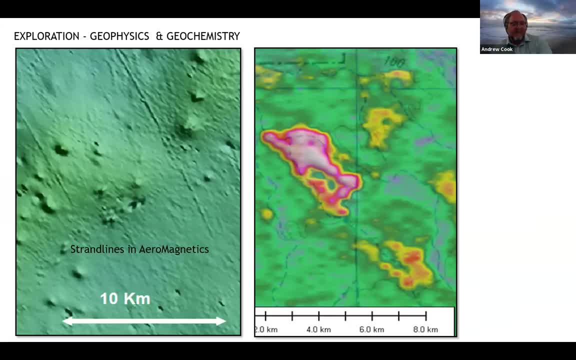 title to, to those areas that look promising. A little bit now about other other techniques that we could use. Well, geochemistry first. Mineral sands is not well disposed to geochemical prospecting. Those minerals being resistate show no chemical dispersion away from them. There's not really any pathfinder elements. 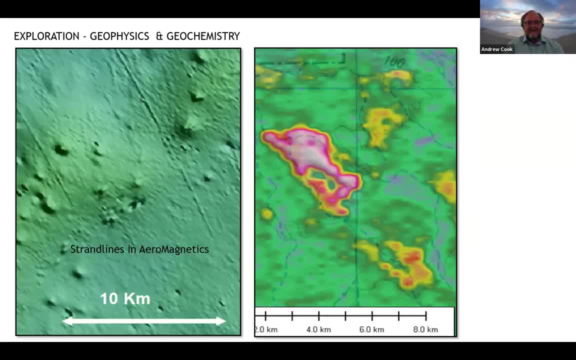 You can detect them directly, but you can't really use geochemistry to zone in on them. Geophysics is much more useful, Radiometrics particularly. It's all centered around the thorium response, which is deriving from the very small amounts of monazite that might be in heavy 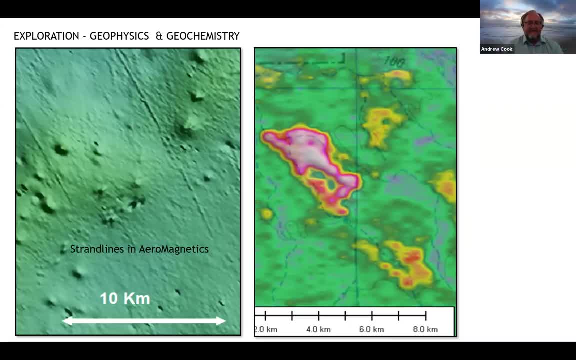 minerals. They can give a very distinct response over an ore body, but they really only work if the ore body crops surface. It only takes a little bit of cover to hide those responses. Aeromagnetics is also useful, Ilmenite being an iron bearing mineral. 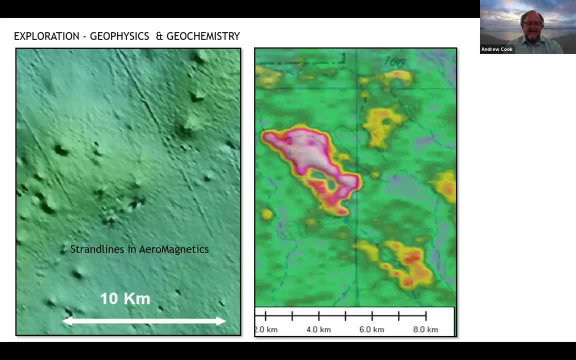 will give a magnetic response, particularly if it's gathered in large concentrations. The grade actually needs to be pretty high because you're usually trying to spot the small response from ilmenite, from an underlying response due to basement rocks, which is typically much stronger And will often drown out your heavy mineral response. 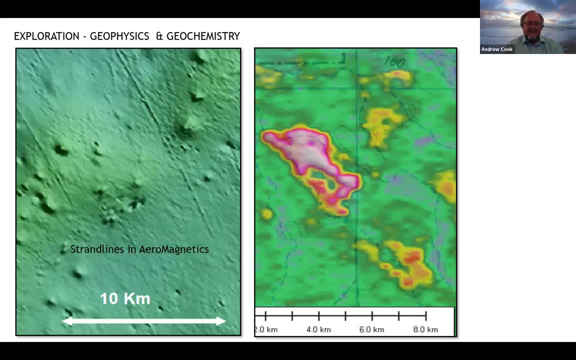 Fortunately, strand style beach deposits are quite straight, and much straighter than than the geology in the underlying rocks, So you can resolve them out by their repetition from line to line in the imagery. Here's an example of a couple of strands in the Murray basin, which is sort of a 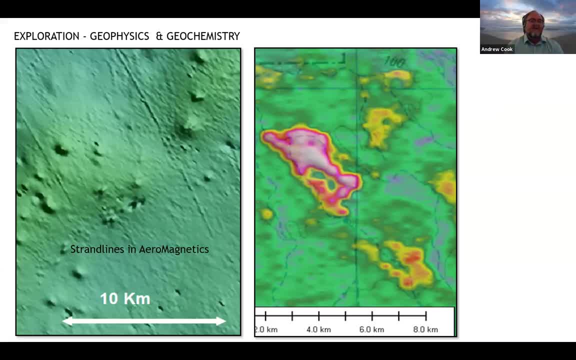 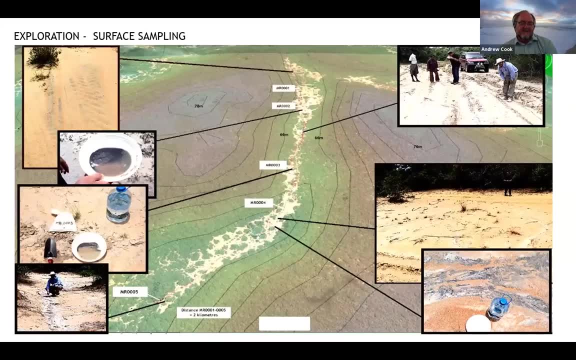 which is an area where the basement is quite deep and quiet, so it's very easy to see the strand line deposits here. Surface sampling, of course, is the other obvious way. Due to surface wash and localized re-concentrations of heavy minerals, you can often find accumulations at surface, and it doesn't take very much grade in the 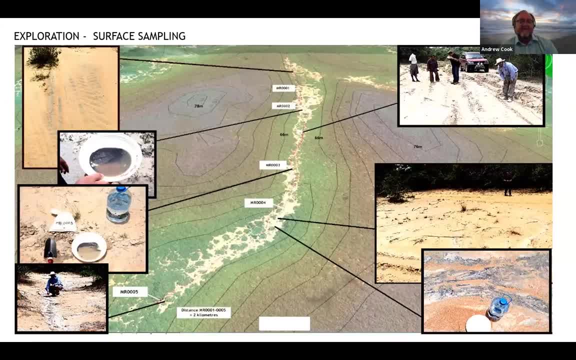 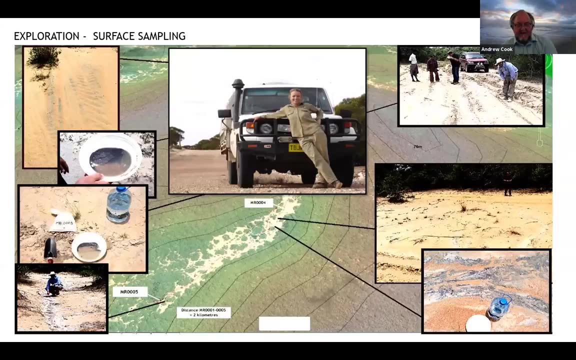 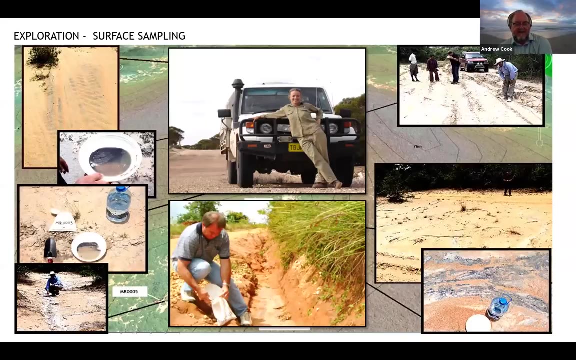 subsurface to create a good showing of heavy minerals in the surface sands, particularly if you have a stream or something washing some material along. We do spend a lot of time out playing around in drains looking for washes of heavy minerals, collecting samples there. 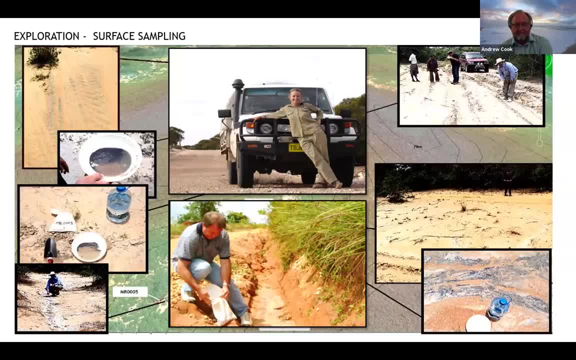 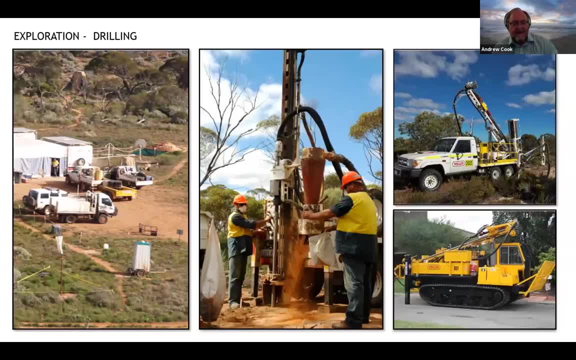 putting our little white plastic pans to good use. Drilling is probably the chief means of mineral sand exploration. Near surface sands are shallow and cheap and easy to drill. Mineral sand ore bodies tend to be pretty large in dimensions, kilometers long and hundreds of kilometers wide. 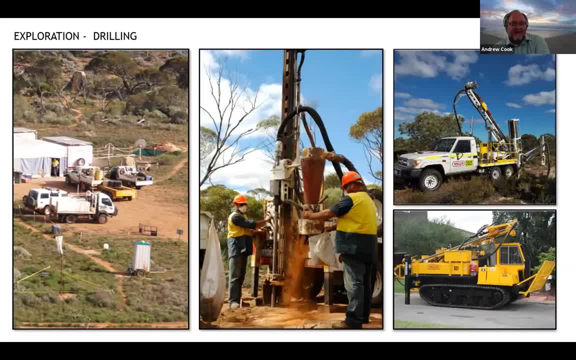 So drilling a series of lines across the country will work effectively to detect these deposits. Air core drilling is the preferred technique. Air core drill bits cut the sand immediately from the face and they funnel it back up with the returning airstream with minimal contamination. 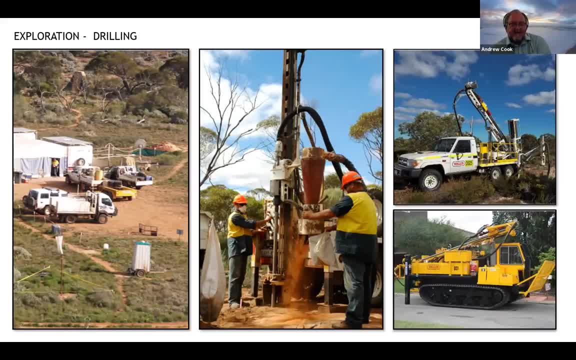 Because mineral sand mines are near surface and open cut, we don't usually have to drill too deep. Possibly 30-40 meters is the minimum. That's all that's required. Most mineral sand deposits can't stand a lot of overburden anyway. 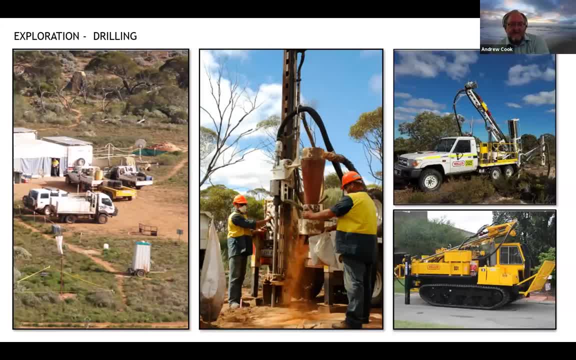 Ratios of less than three to one are preferable. Richer deposit: you might be able to be mined as deep as maybe 60 meters and with ratios of, say, six to one We will collect samples down hole, Usually for exploration. you might start with a two meter. 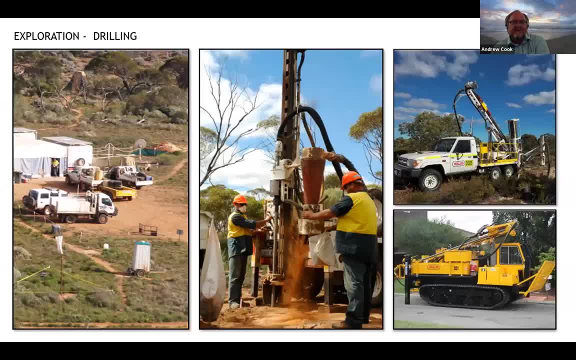 sample interval, but anytime you're measuring ore- probably one meter- You can see a rotary splitter here below the cyclone and samples being split into those. one or two kilograms is normally collected And a couple of drill rigs. these both belong to Wallace Drilling. 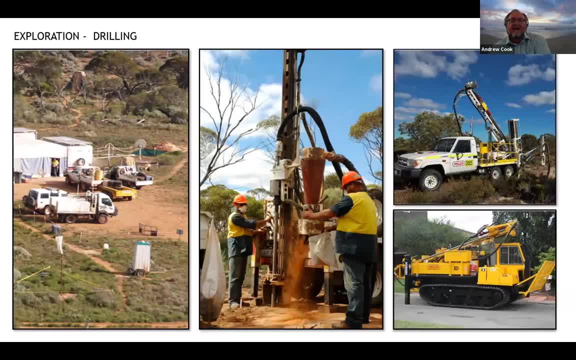 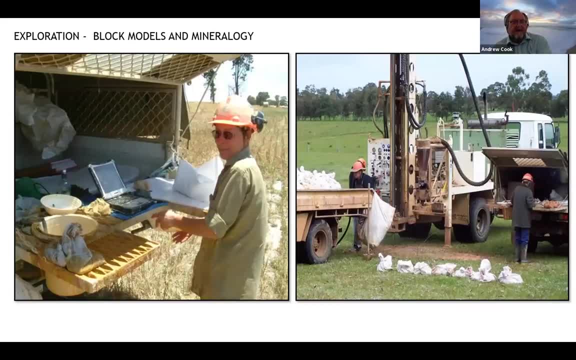 the inventors of the air core system. They're quite small and mobile and easy to get around. So here's a picture- an older one, an older picture- of a geologist working on the drill rig. I thought I would just let you know the sort of information that's recorded. 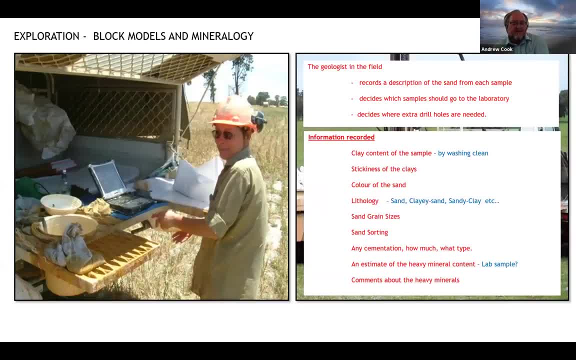 There's estimates of the clay content of the sand, how washable it is, how sticky it is, how much is there maybe the grain sizes of the sands, the grain sizes of the heavy minerals, any induration or cement that might be present? 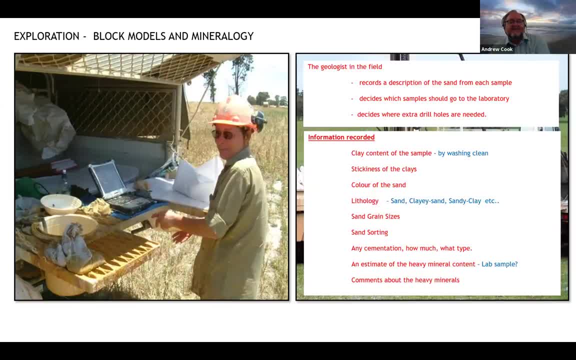 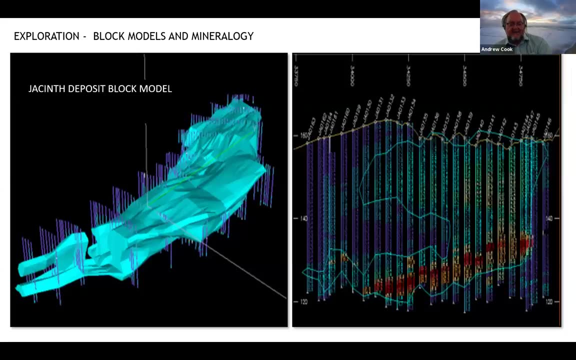 Geologists will quite often also try and make a guess as to which facies they're in. You might log it to say you know dune sands or shoal sands. And it's pretty important that the geologists get a good understanding of the ore body because 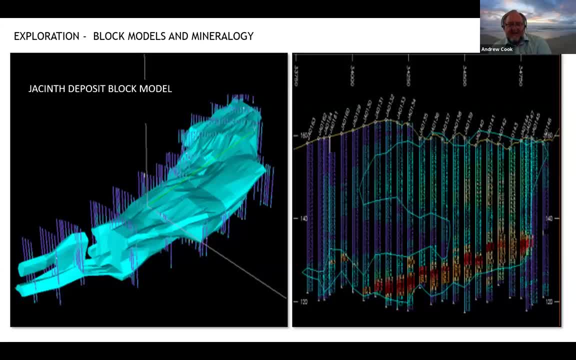 discerning those facies is very important In determining the mineralogical variation throughout the ore body. and these have to be determined because when you go ahead and create your block model ore body, the grades that are in it have to be informed of the changing mineral assemblies throughout. 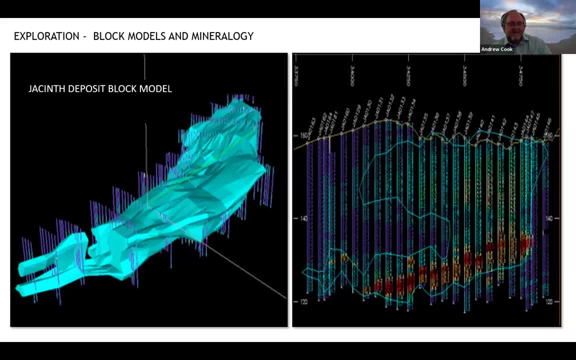 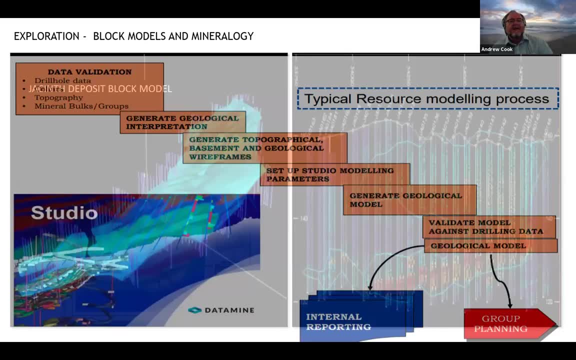 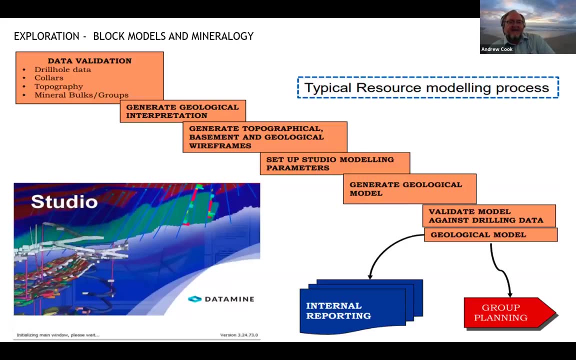 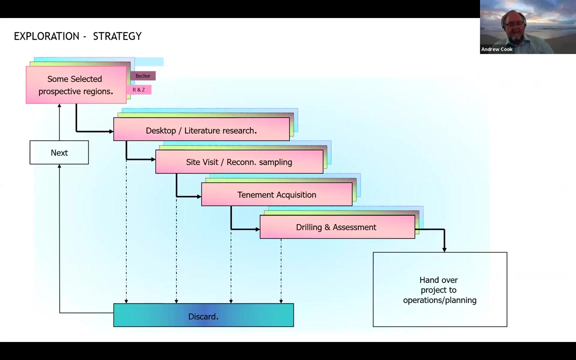 the deposit so that the proportions of different minerals in each area can be worked out. There's quite a focus on block modeling and integrating mineralogy. This is a sort of flow sheet of the typical process. So the drill test evaluation of these paleo shorelines. 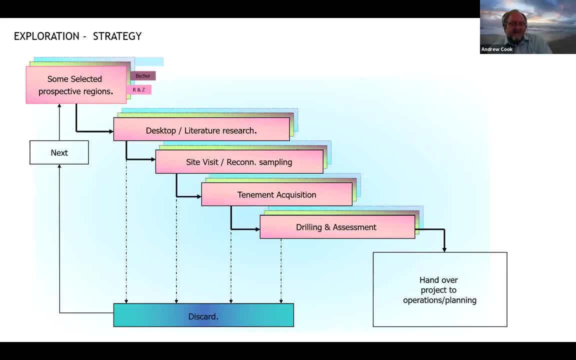 exposes a range of deposits of varying grades, and companies like Iluka usually maintain an inventory of resources. They might not all be economic at the time and it's usually important to try and exploit these deposits sequentially as you open up an area. So the establishment of 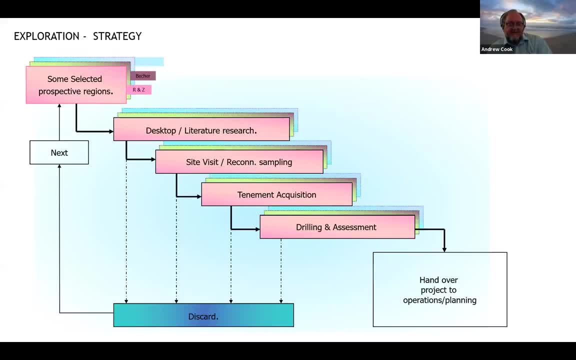 the infrastructure to operate these deposits is important To process. one deposit can suddenly lead to a bunch of lesser lights in the vicinity also becoming economic. So basically, though, for a deposit to have immediate impact, it will need to be amongst the best that's available at the time. This will supplant others, may become the